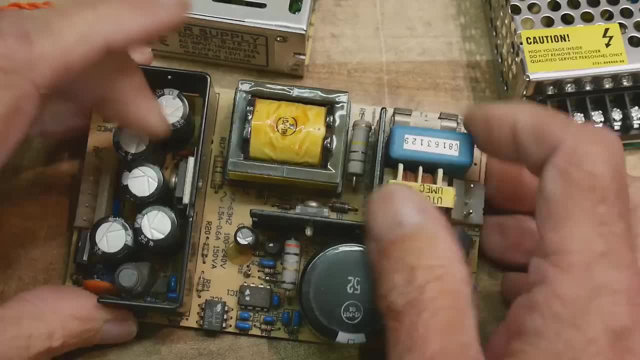 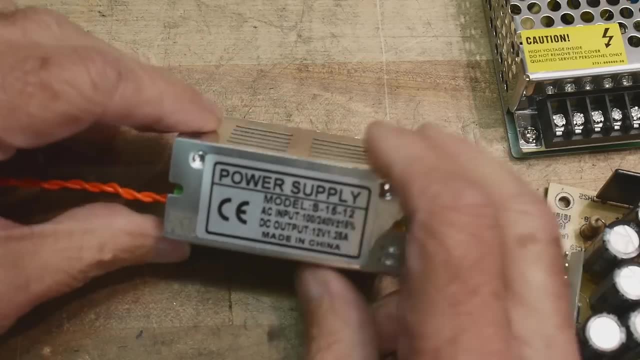 So it's got a lot beefier components, It's got a fancier input section and stuff, But the way that this operates is going to be exactly the same as the way we have it pretty this operates. So let's get started, Let's open this thing up and and see. 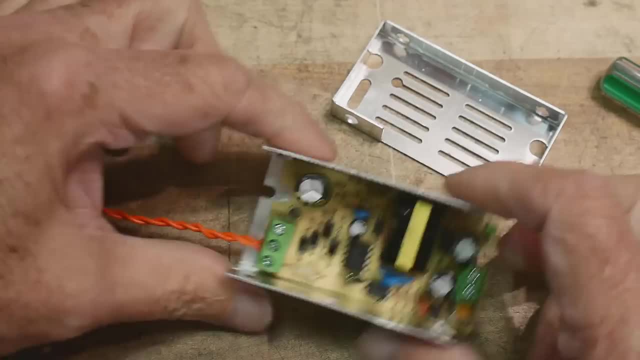 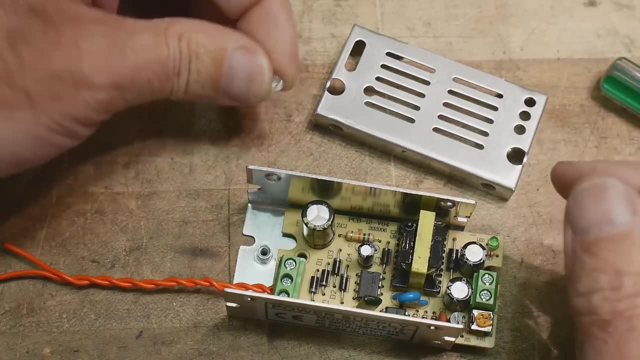 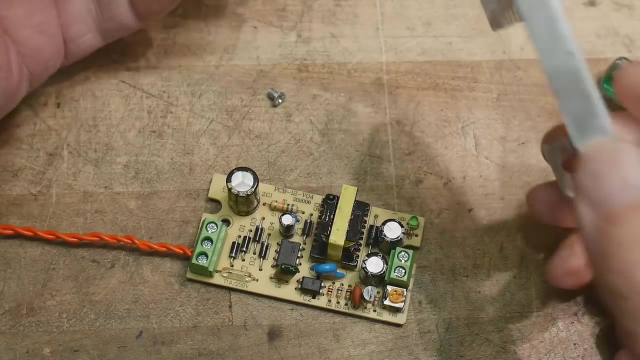 what's inside. Okay, so the the top just pops off, it's just held in there by friction, and then there's one screw and you take that screw out and then the circuit board will come out. Okay so this is all just a metal and it's not used as. 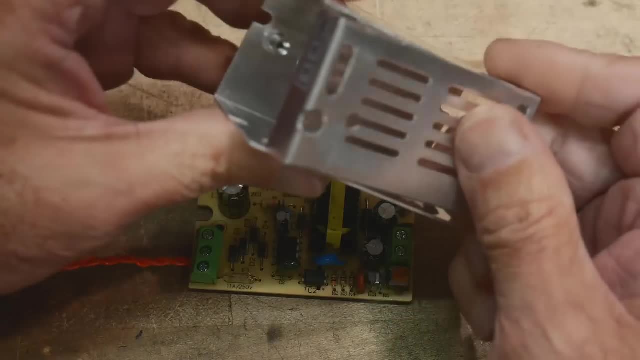 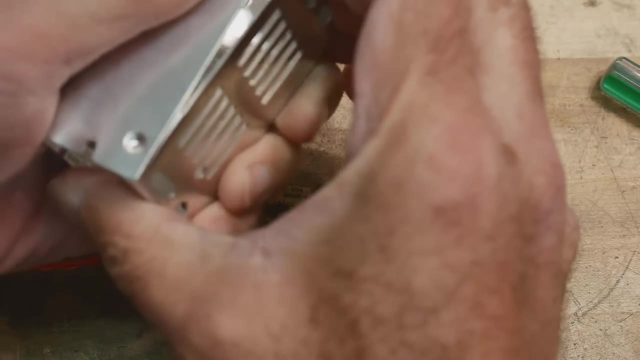 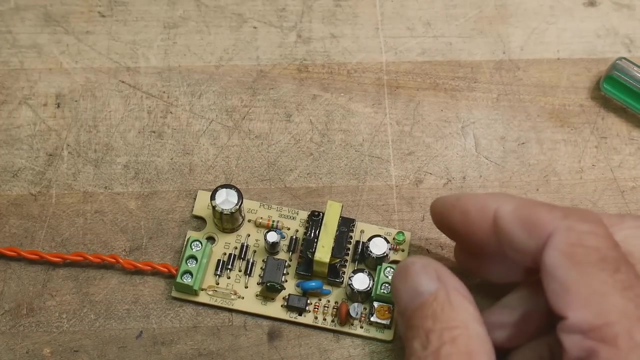 a heatsink. It doesn't do anything at all. It's just a RF shield, I suppose, and more importantly, so you don't get your fingers in there and get electrocuted. So so this is the board. Let me, let me get rid of these things, All right, so this is. 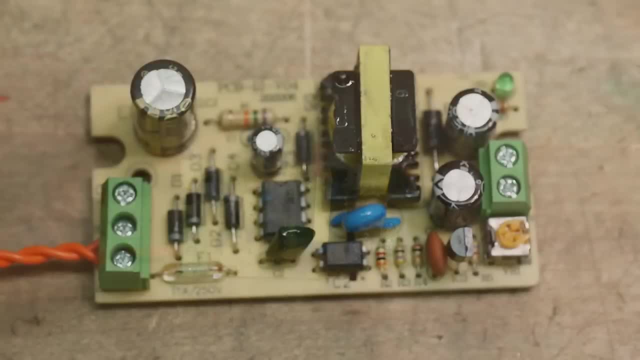 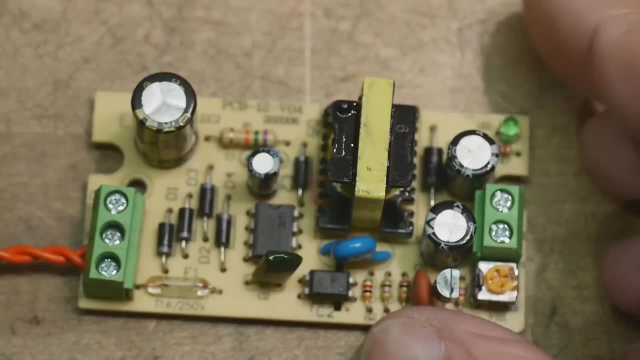 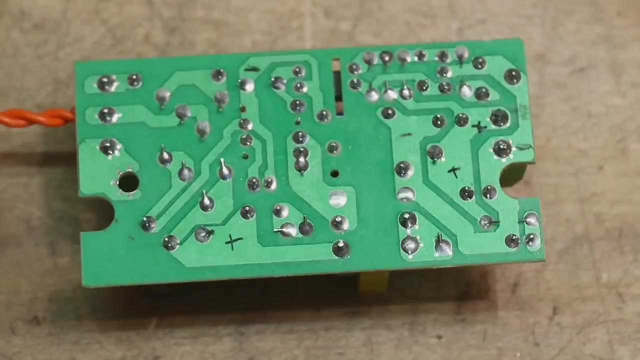 gonna be the circuit board and it looks pretty simple. That's strange. my camera, my camera timed out. I don't know why it shut down. Anyway, Let's, let's start drawing the circuit. There's not much of the PC board, It's a. 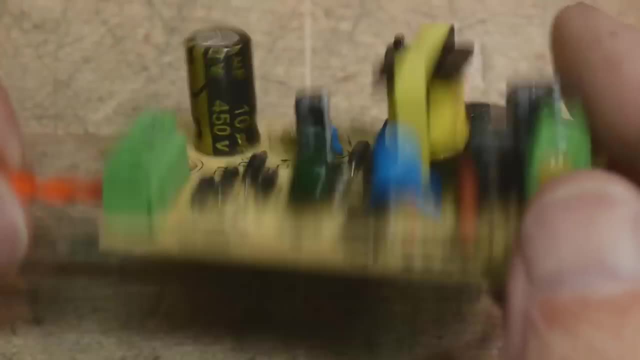 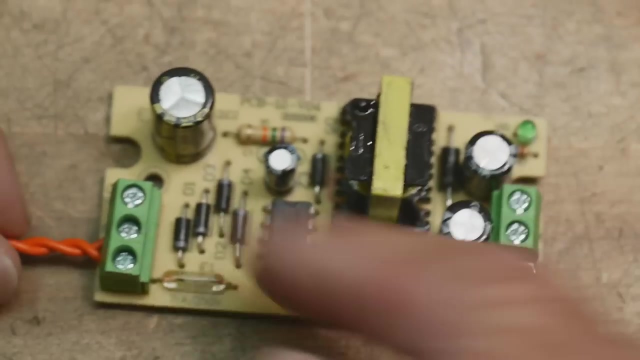 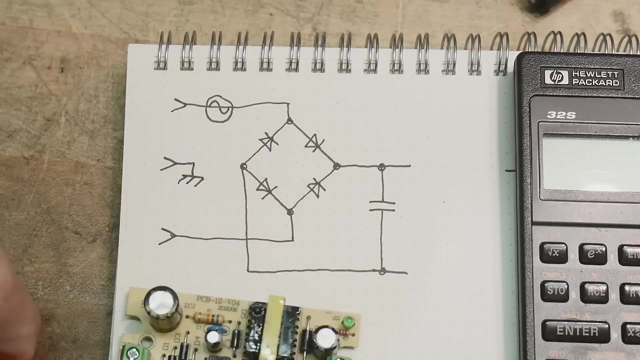 single-sided PC board so it's easy to see the traces and easy easy to see where things go. So let's start, let's start drawing a schematic for this thing and then I think we'll have a better understanding of how things get from one side to the other side. Okay, let's take this a step at a time. So I've 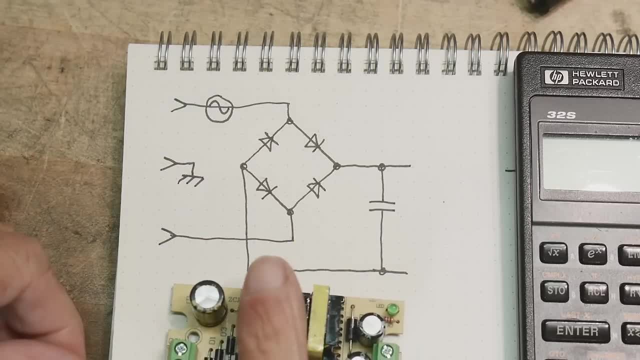 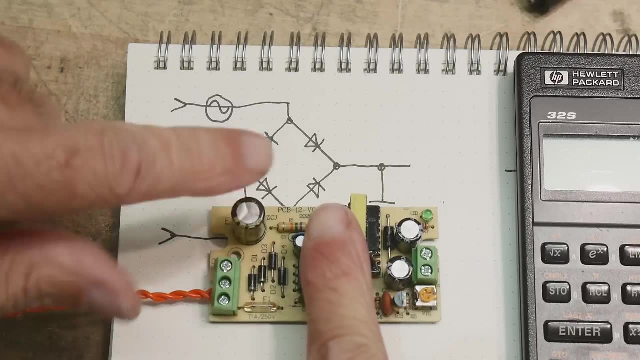 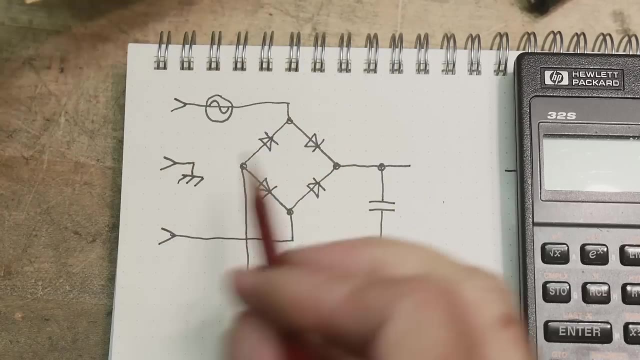 traced out the front end of the circuit board and then I'm going to take this out of the circuit. about that much of it. Okay, the bridge rectifier and this capacitor and the fuse and then the connection here. Okay, so that looks like this: The AC comes in, it goes into the bridge rectifier, All of the, all of the. 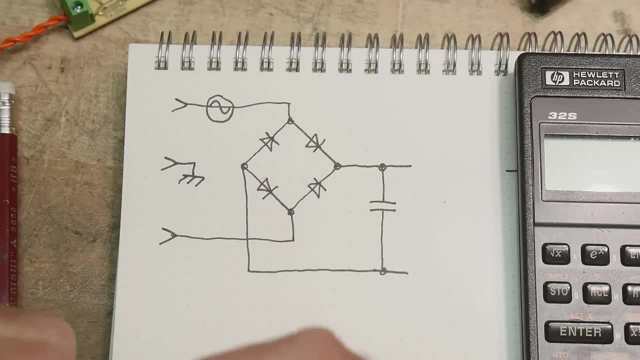 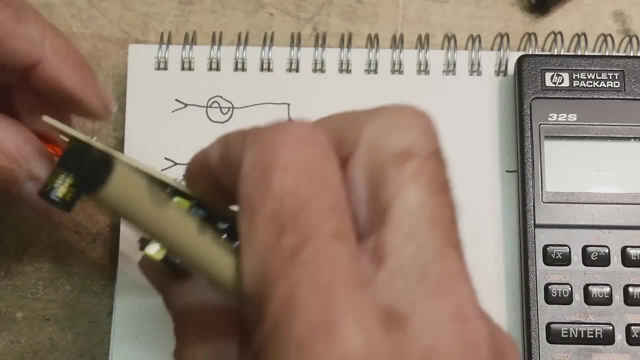 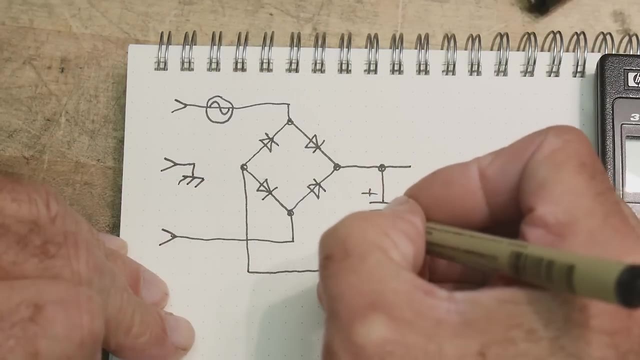 positive things go in the positive direction, all the negative things go the negative direction. So we end up with this capacitor here and we have a pretty nice capacitor. let's see what value it is. It is a 10 microfarad, but at 450 volts, so lots of volts there. So let's. 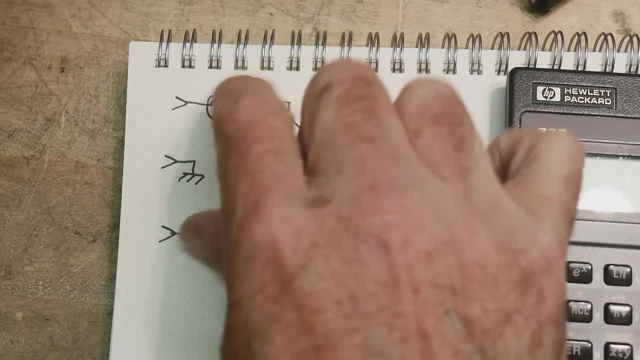 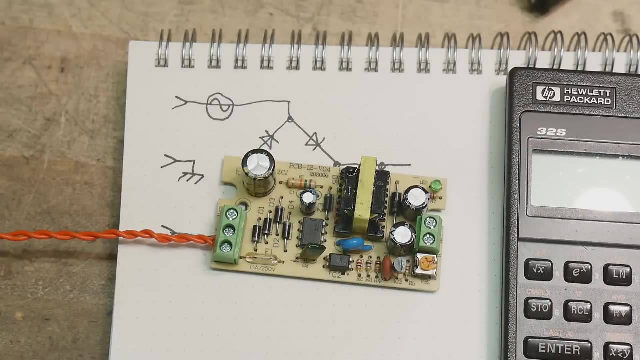 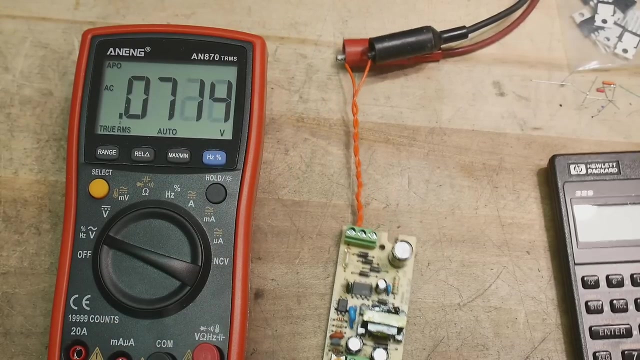 go ahead and turn it on. Let's measure the voltage that we get here. We can measure the AC voltage coming in and we can measure the DC voltage coming out. okay, So let's go ahead and do that. Okay, let's, uh, let's turn it on. We do get a, we do get a green light. you can just whoops, Let me move. 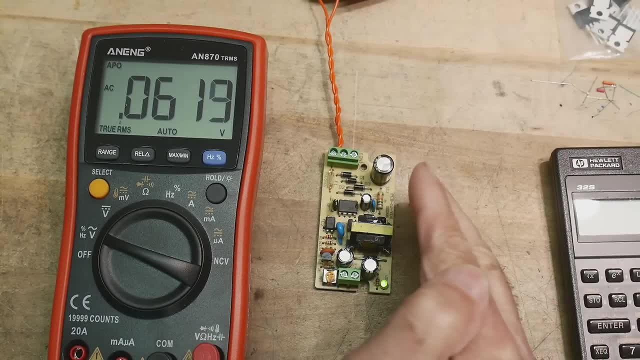 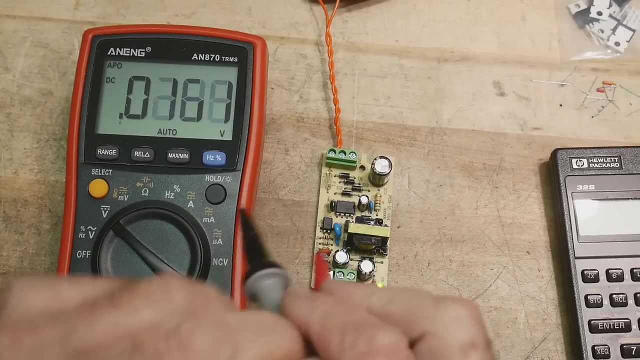 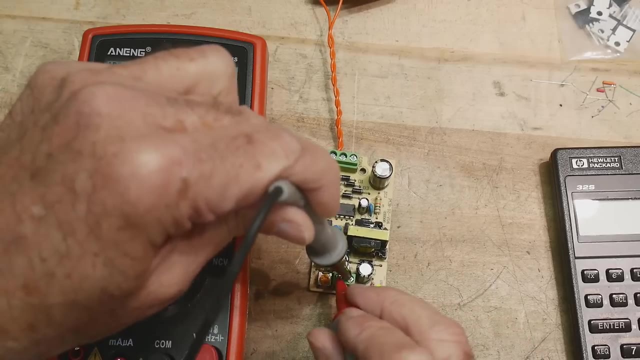 this up. I think you can see the green light down here. so it is working. And in fact, let's measure the output. since we're here, Let's go ahead and measure. measure the output and we're getting twelve Volts out. Twelve- uh well, I guess minus around this direction We're getting. 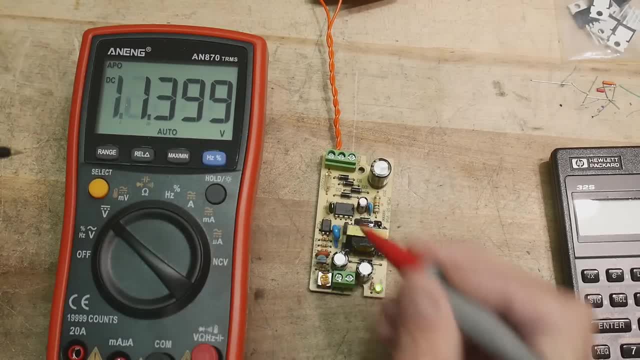 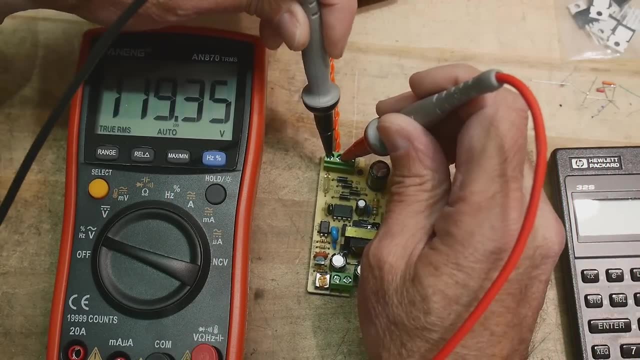 twelve Volts off, 12.1 volts out. that's good, Okay. so let's take a look at the input. We'll go to AC on our meter. We'll measure the AC, so be careful about this. So we're measuring 119.4 volts input. 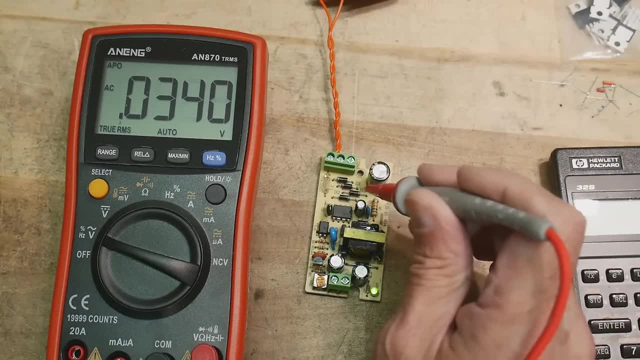 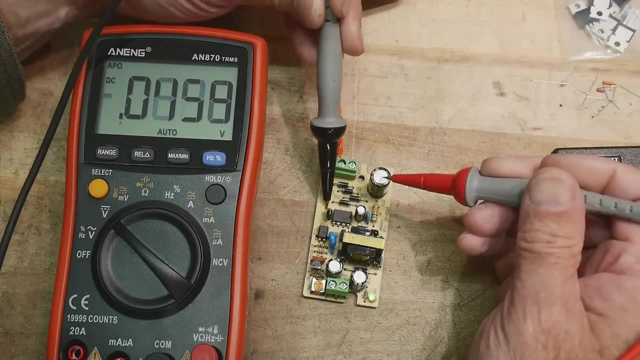 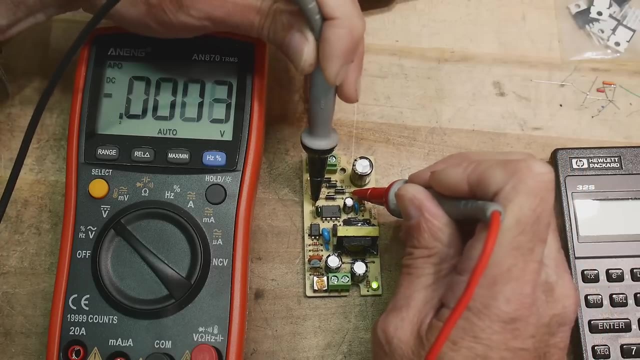 so that's the AC coming in And then it's gonna go through this bridge rectifier and it will get rectified. so we'll go to volts And I know that ground is right here and plus is right here And I don't want to zap myself. 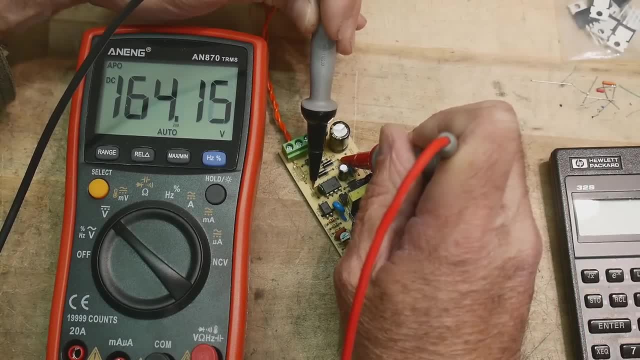 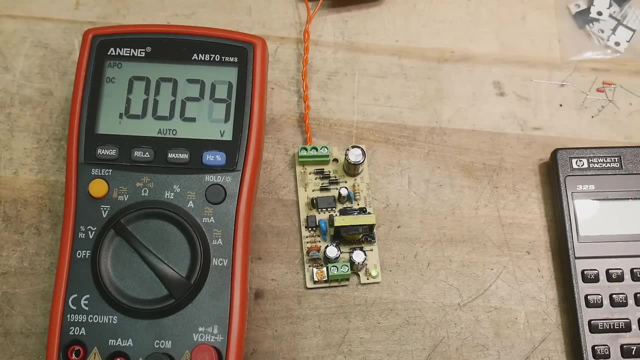 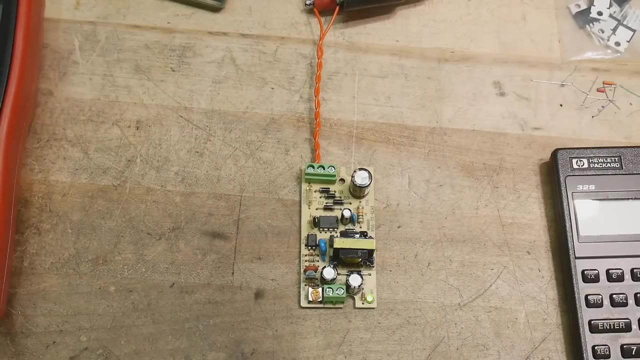 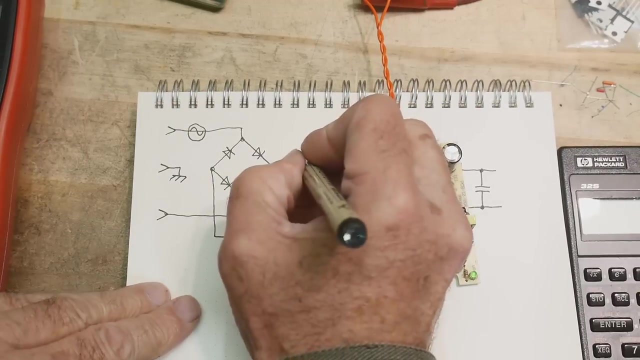 There, So we are measuring 164 volts. okay, 164 volts, All right. so let's write a couple of these things down. Turn this off so I don't zap myself. All right, so we have 164 volts Volts DC. 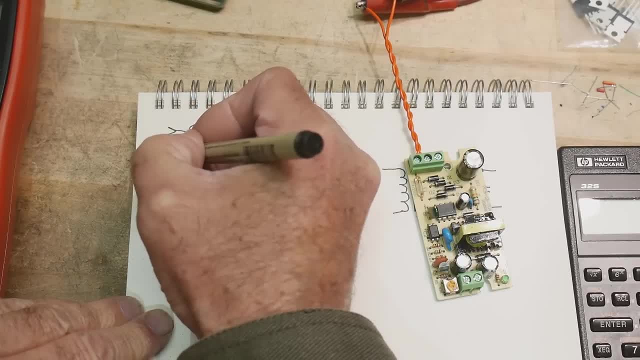 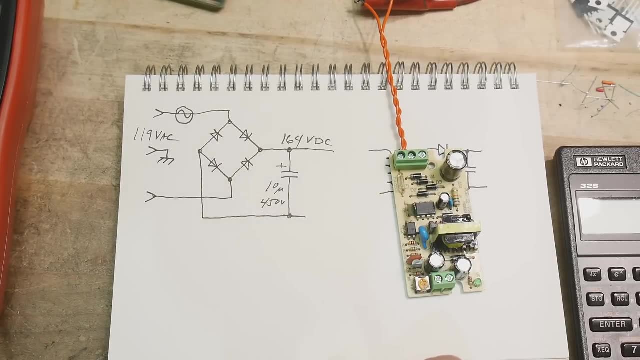 We had 119 volts AC coming in. All right, so 164 volts, All right. so the next thing we're gonna do is we're going to take our AC. we turned it into DC. now we're gonna take the DC. 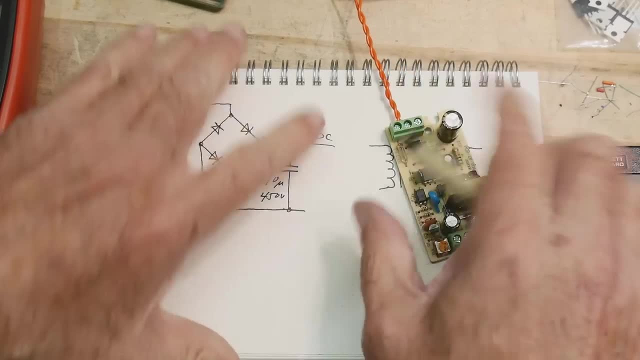 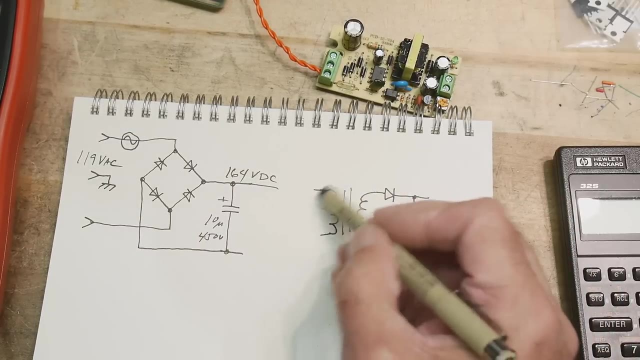 we're gonna turn it back into AC again, okay, Okay. So the next part of our circuit now looks like this: okay, It's a transformer, so we have AC on this side, which means we have AC on this side, and then it gets rectified. 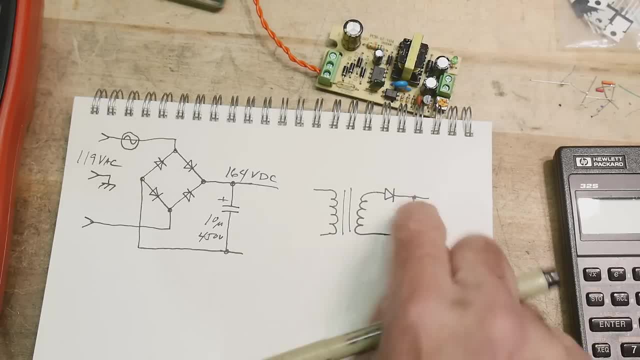 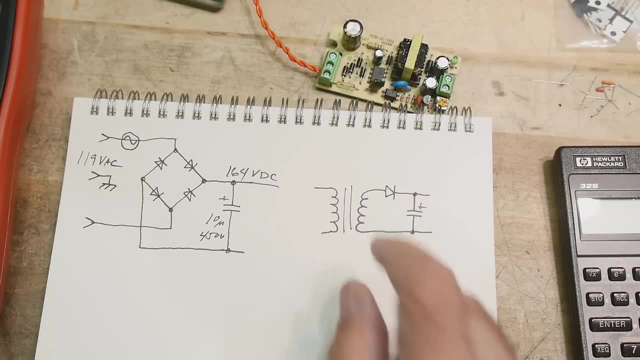 Instead of a fancy bridge rectifier, it's just a single rectifier and we will have a DC voltage again. all right, And so how do we generate AC volts here Now, if you watch my series on DC to DC converter, okay, 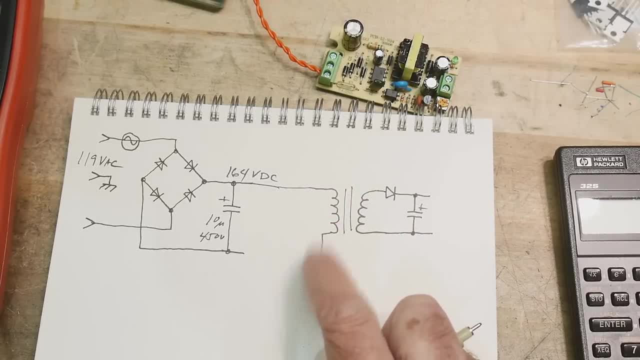 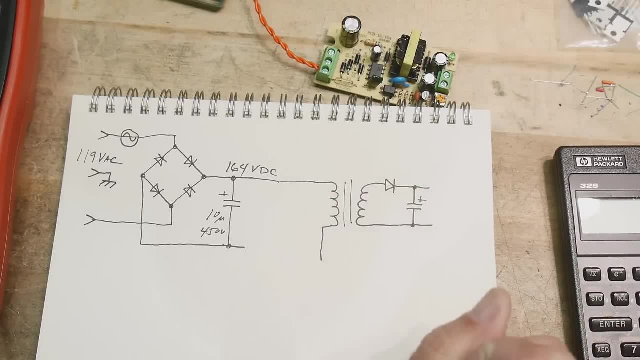 which would cause an alternating signal here, which would get rectified and cause a DC over here. All right, so how do we do this? Well, we're gonna use a fancy chip, okay, And so we have it. We have a fancy chip to do that. 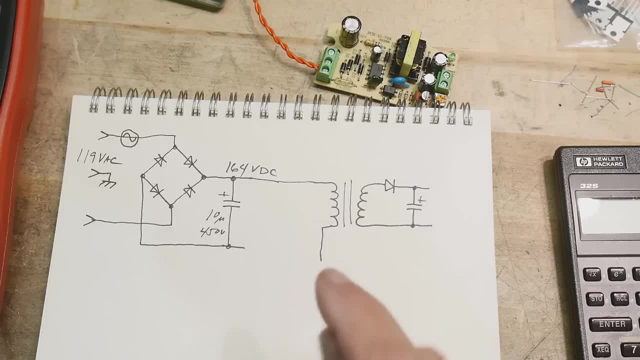 I won't draw it in yet. One of the things, though, that the circuit has that we have to explain is, whenever you have a coil and you let it go, it's going to generate what's called back EMF. It's gonna generate a negative pulse. 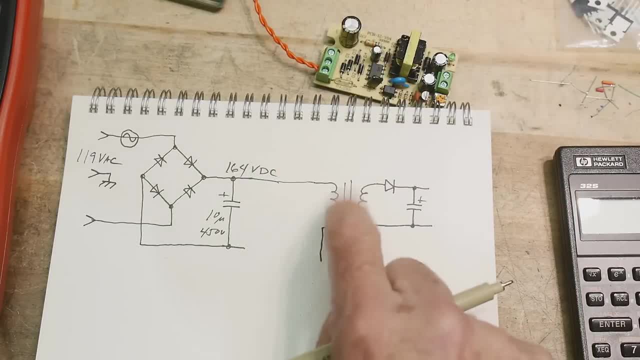 Remember when I did the tap, tap, tap, it created that big spike. Well, we're gonna get a spike here, We're gonna get good current flow, but then when we release it, we're gonna get: whew, we're gonna get a big spike. 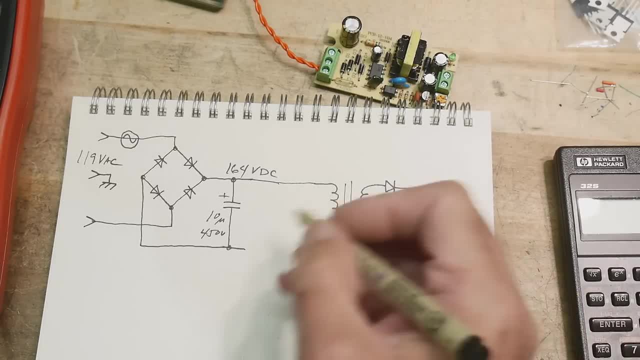 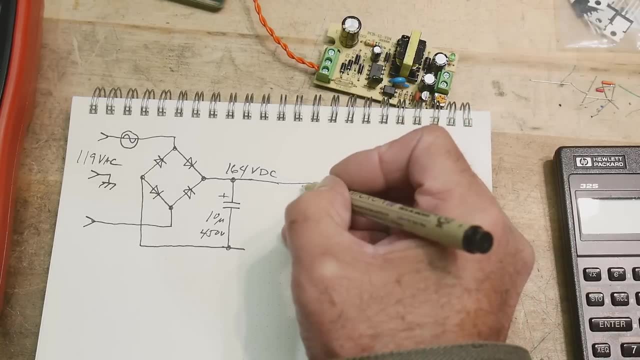 And we have to. we have to kill that spike and we're gonna put a. a lot of times you'll see this off of on motors or on solenoids and stuff on relays. Very often you'll have a diode. 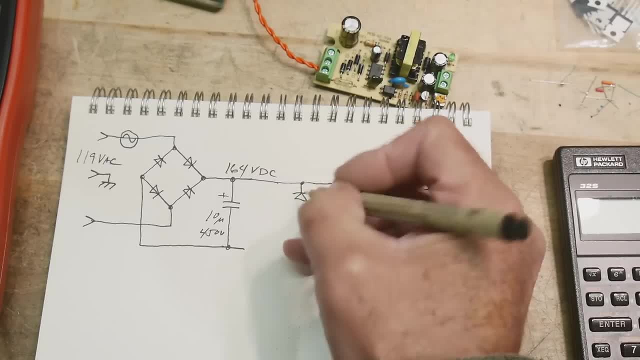 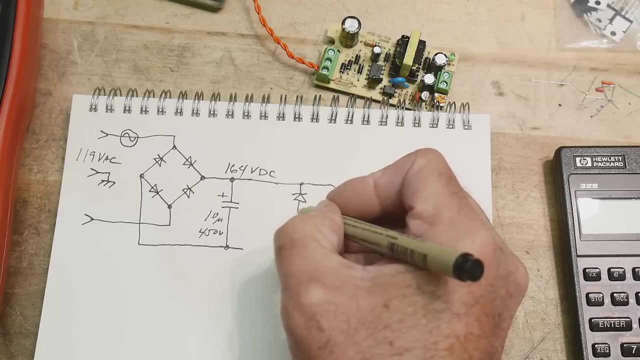 a reverse diode across the, across this winding. Now they do have a diode in there, but they made it a little fancier. They went ahead and they put a resistor here too to limit the current okay, And so they have that going, that going across. 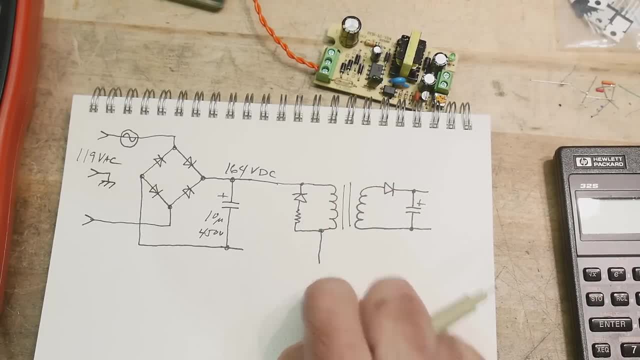 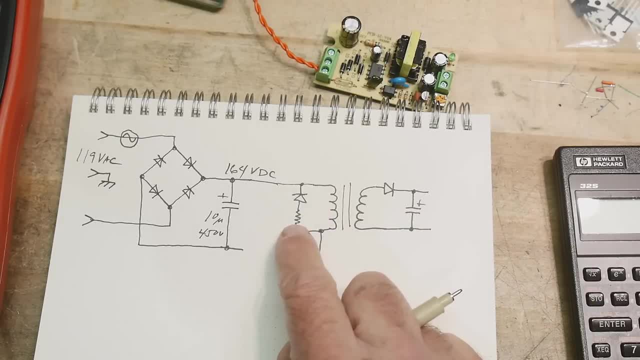 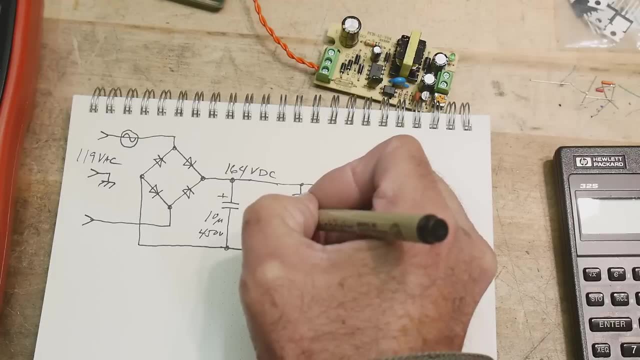 And they said: well, we want to limit the current, but we don't want to slow it down, And so we're going to put a capacitor here that will be really good at taking off the edges. It will allow large currents to flow. 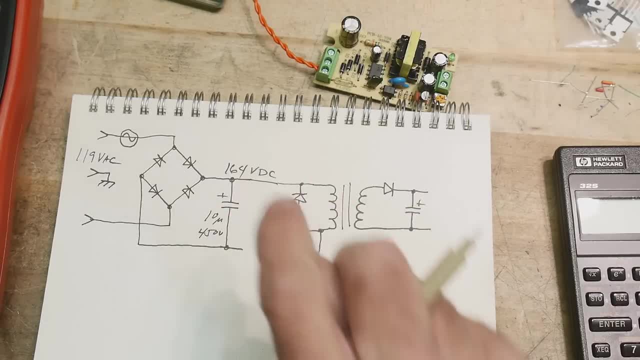 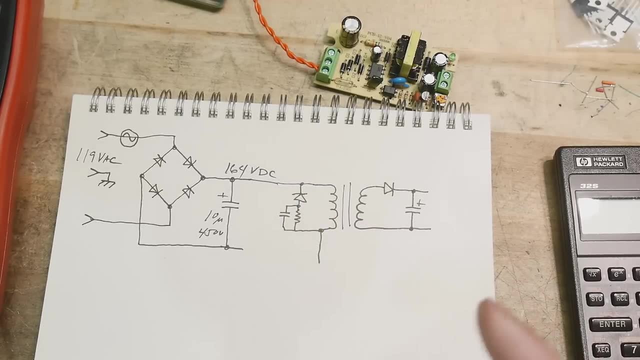 but only on really, really high frequencies, only on that sharp edge. As soon as we get rid of that high frequency, sharp edge, we'll let this resistor do its job. And this, this will be our next step, This will be our snubber circuit right. 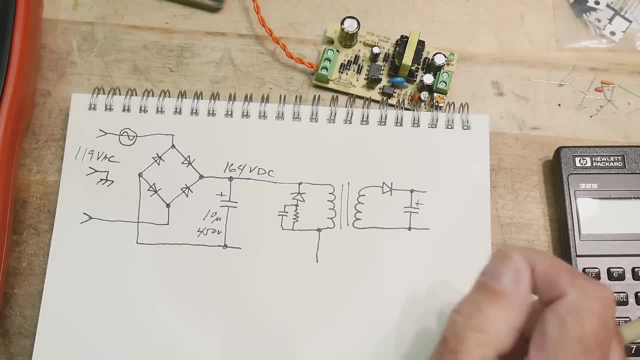 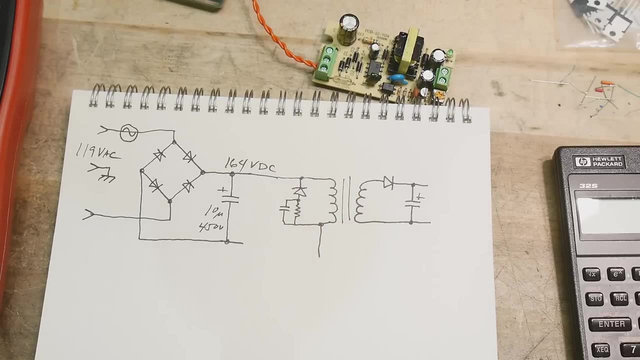 So that's what they have in there. So that's what. that is All right. So now we need some way of tying this to ground and pulsing it on and off, okay, And so if we take a look at our circuit now, we've explained. 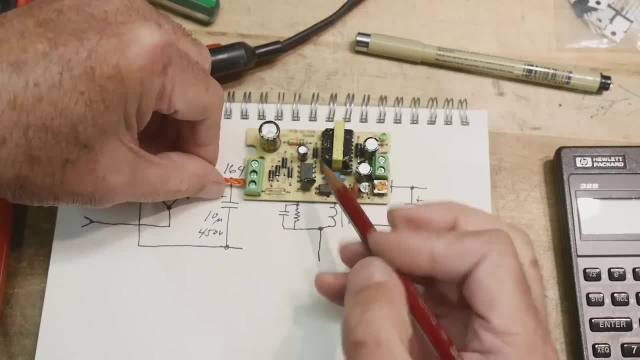 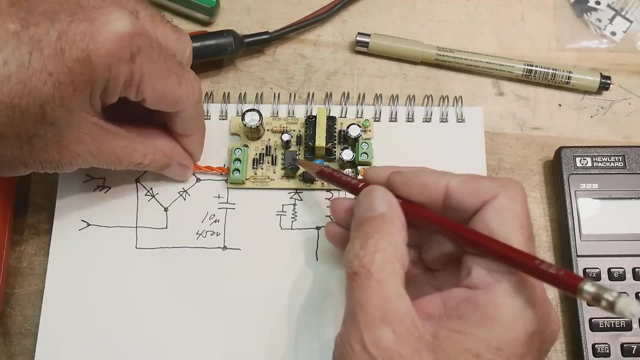 where's my pointer? We've explained all of the input and we've explained the snubber circuit over here, And now we end up with an IC. There's an eight pin IC here And here's our transformer- okay, The transformer's here. 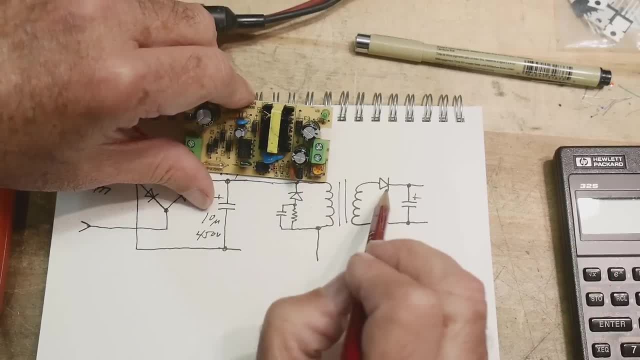 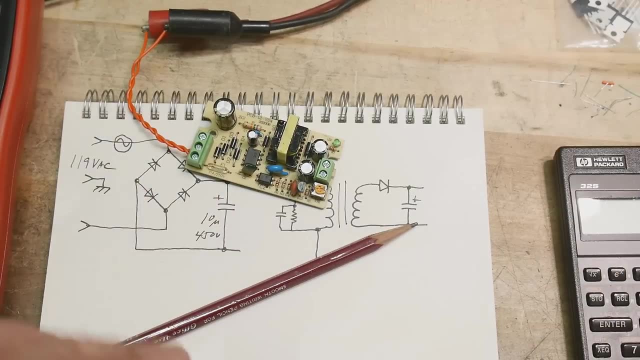 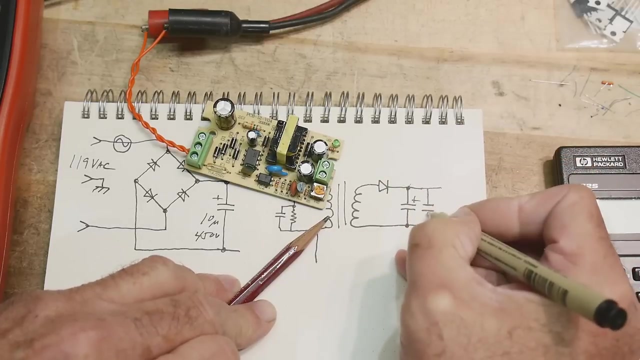 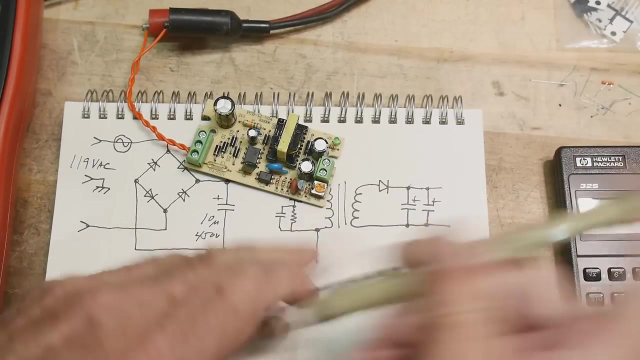 The transformer has its diode, which is down here. That's this diode, And it has its capacitor, And in this particular design, it actually has two capacitors. So they did that to make the capacitor bigger, right? So that's what. that's what we're going to do. 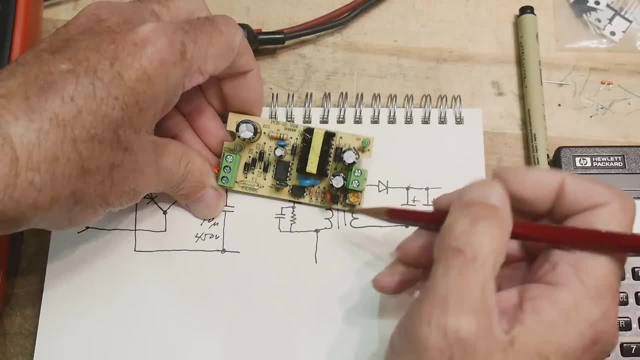 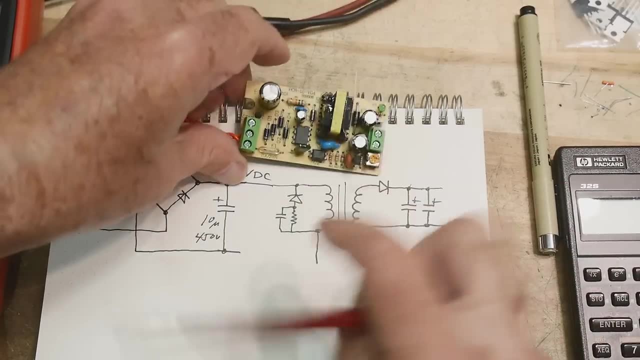 All right, So that's what these two capacitors are. These two, here are those two, So we almost have the whole thing already. but okay, So we have an IC that's going to do all the magic. The IC is going to have an FET on it that does the pull down. 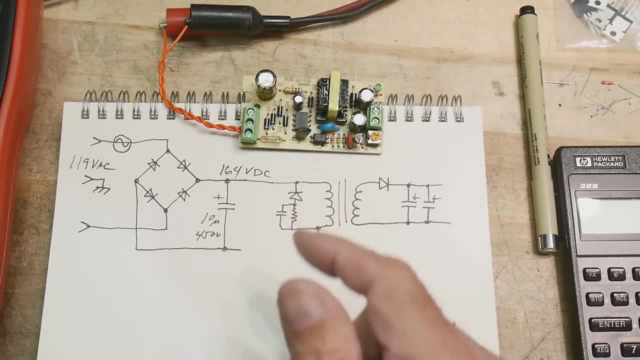 It's going to be pulsing this thing, But it also is going to have the feedback loop And it also is going to have the oscillator. Remember I had a 555 timer that was going tick, tick, tick, tick, tick, tick, tick. 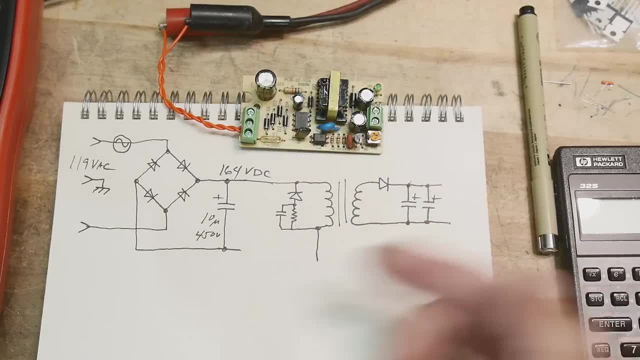 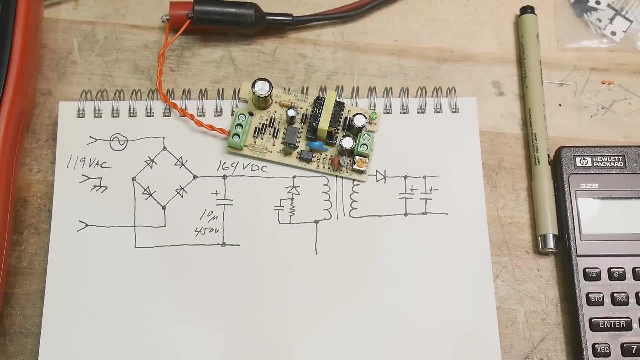 And then we had some circuit that said, you know, don't tick or tick right, And we had some kind of feedback And that's all going to happen. And this IC, so this IC- is made for this purpose. So let's go ahead and draw that in next. 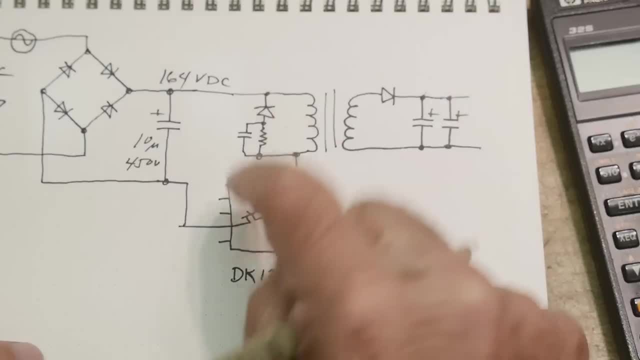 So I've drawn in the circuit. It's an eight-pin device. Okay, So this is pin 1, 2, 3, 4, 5, 6, 7, 8.. Pins 7 and 8 are tied together. 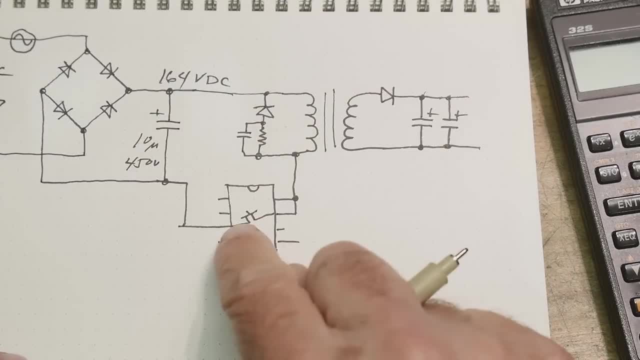 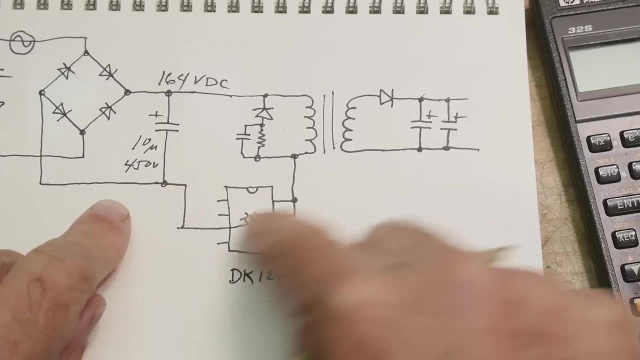 And they have this FET that's inside And that FET is going to pull down on this coil and to ground, So it's going to complete the circuit right. This will be the circuit here And it will go: tap, tap, tap, tap, tap. 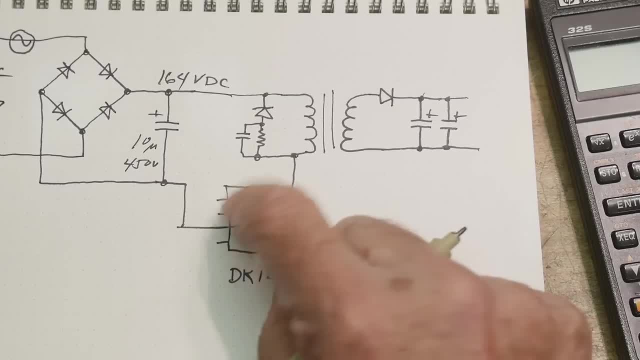 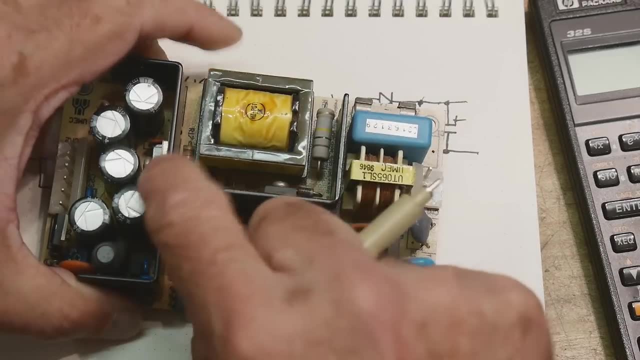 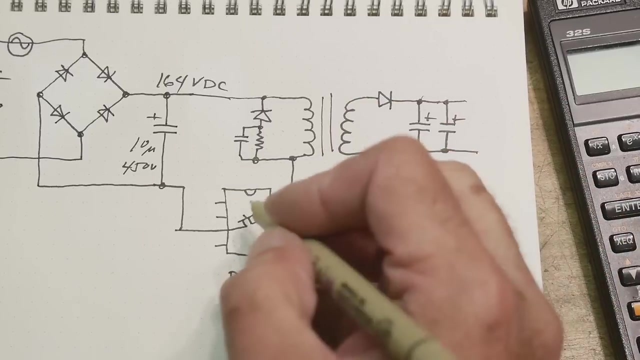 So this will be doing the tapping, this built-in FET. Okay, Now some power supplies like these big, beefy ones. they'll have external power transistors because they're really, really big and they need to be big, But this one, this is good enough for one or two amps. 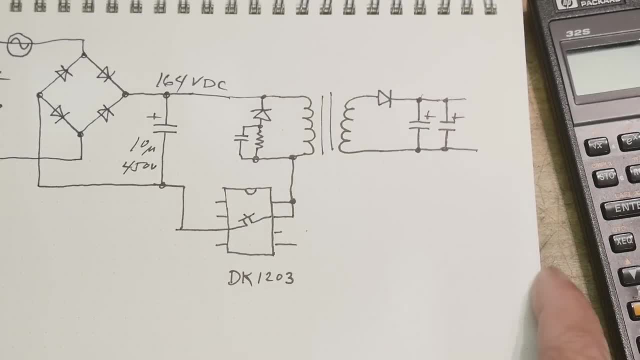 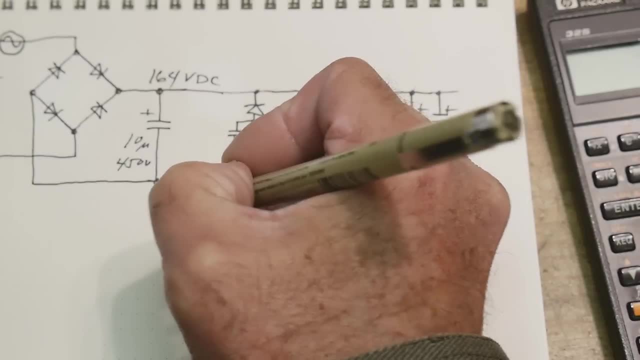 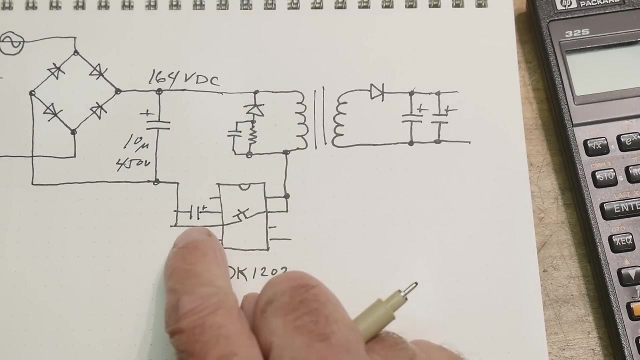 And so it's built into the IC. But it has that transistor in there. Okay, It also has the oscillator. It has a whole bunch of other things. Now, to make this thing work, you have to put a capacitor here, And then the only other thing is this pin. 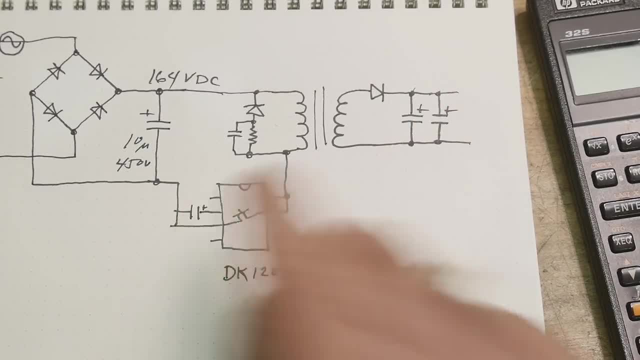 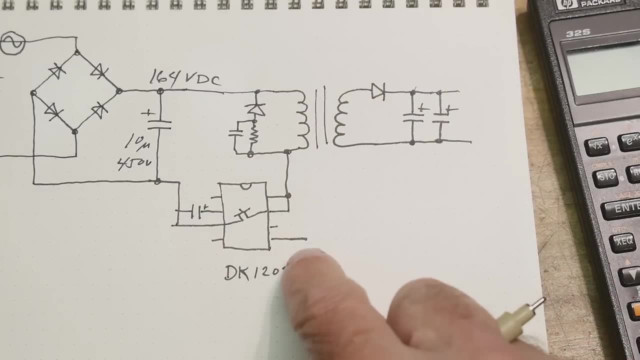 So this is not used, and this is not used, and this is not used, But this is going to be the feedback. This is the one that tells it whether you're too high or too low. That's going to be our feedback, So we'll draw that in later. 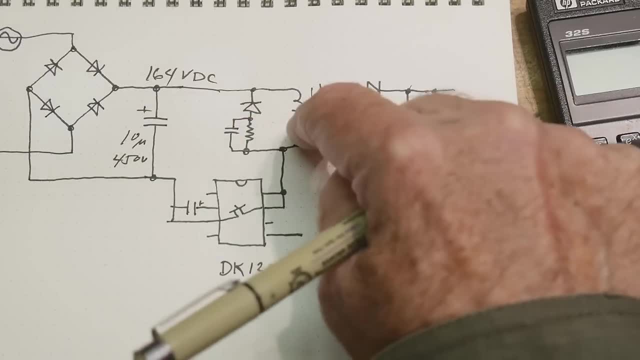 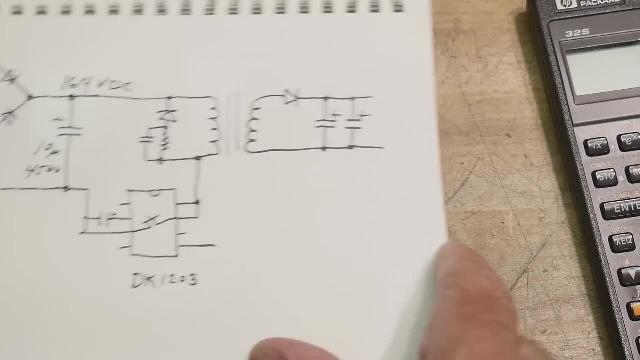 But you get the idea now That we have DC and now we're going to turn it back into AC by having this transistor and going tap, tap, tap, tap, tap, tap, tap, And then we're going to then turn it back into DC again this way, 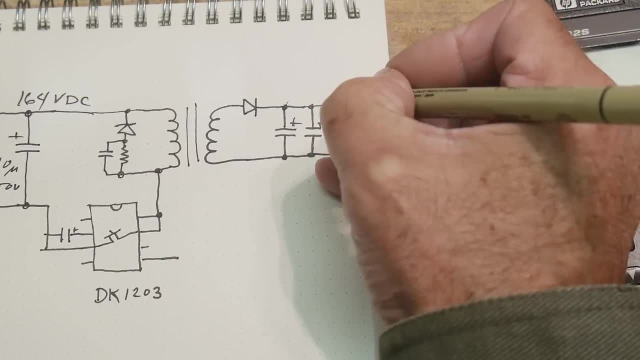 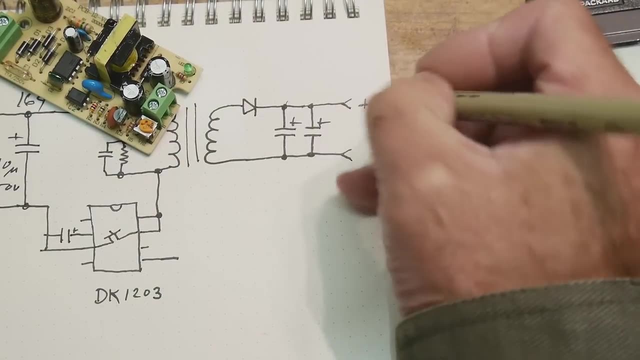 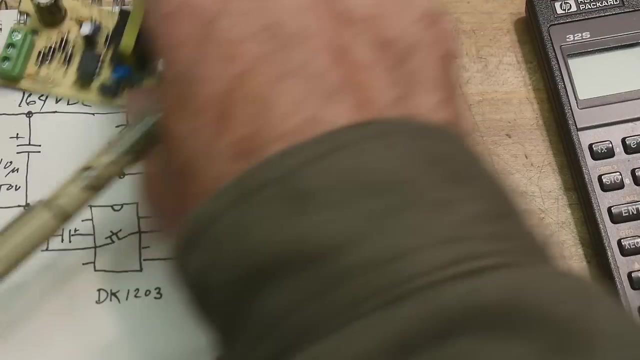 And these will actually go to the outside. So that is actually this little green connector on the back And this is our plus connection and this is our minus connection. So this is where we're going to get our 12 volts- 12 volts over here. 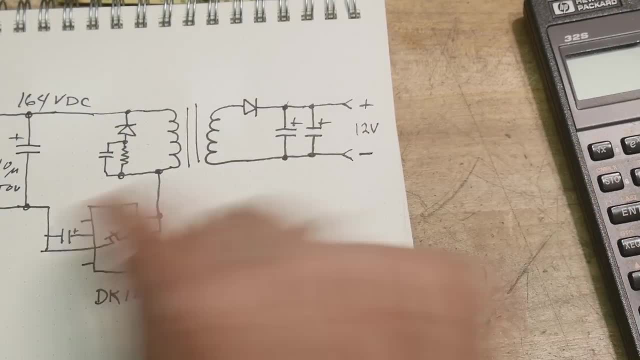 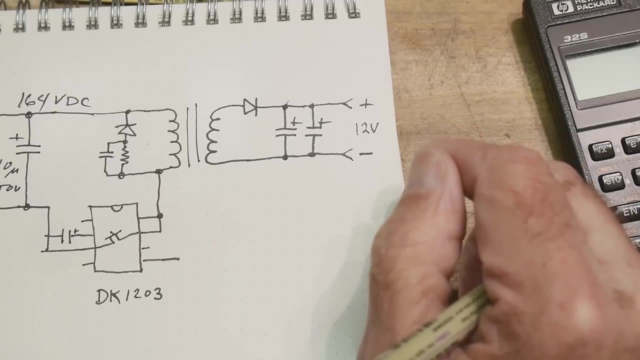 All right, So we basically have the whole circuit now. There's very little else except for this feedback. Okay, We need to figure out how to do this feedback And we have to be very careful because we have really high voltage things over here. 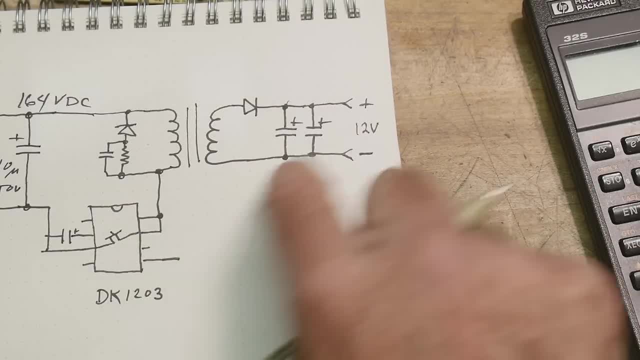 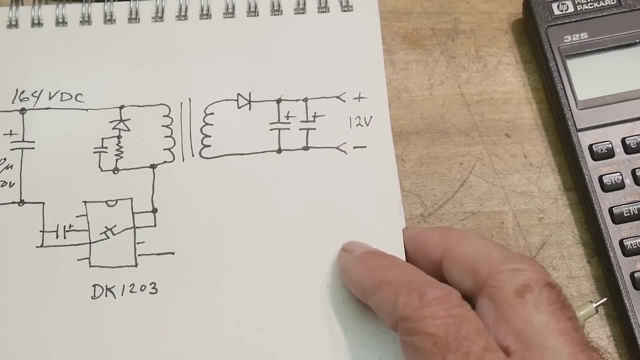 We have very low voltage things over here, So we don't kind of we don't really want to connect them together. Remember, this is 164 volts over here And we want to, we want to isolate those, So we want to isolate those. 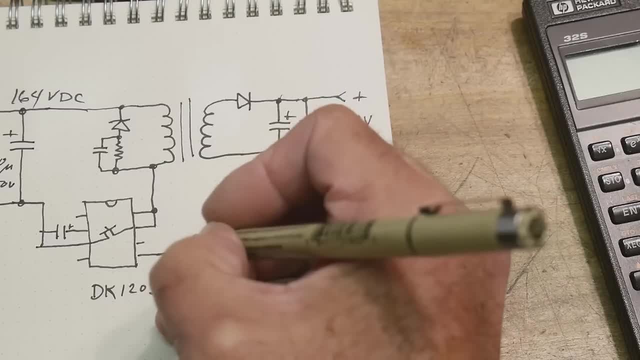 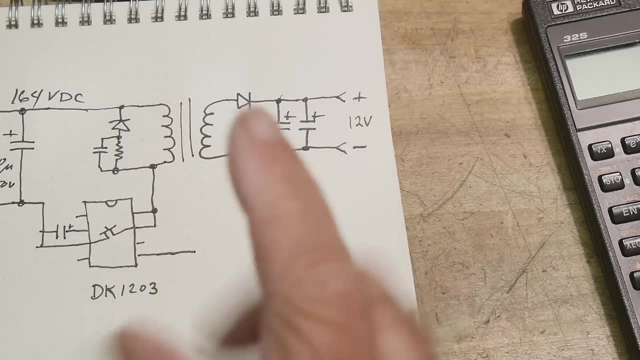 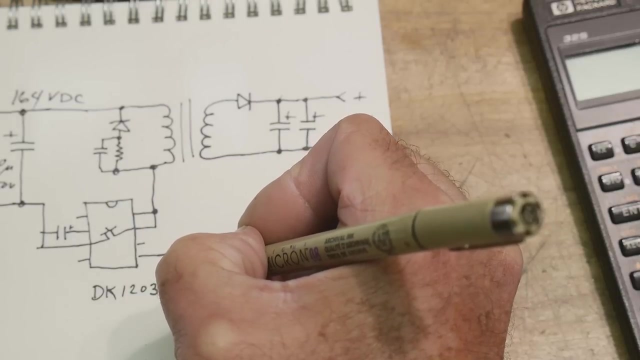 So how do you isolate something? Well, you can use an optocoupler. Okay, So this here. what it needs to do is you need to pull down on this wire in order to regulate, And so we're going to come and we're going to put in a transistor. 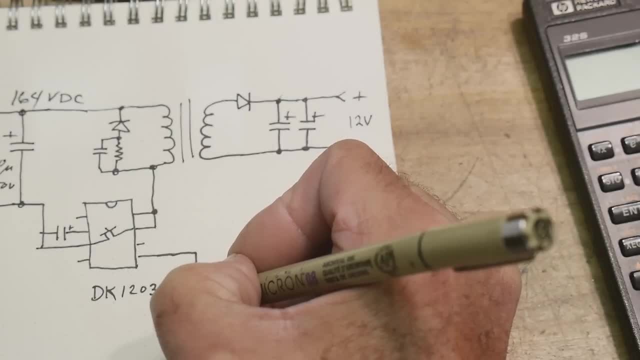 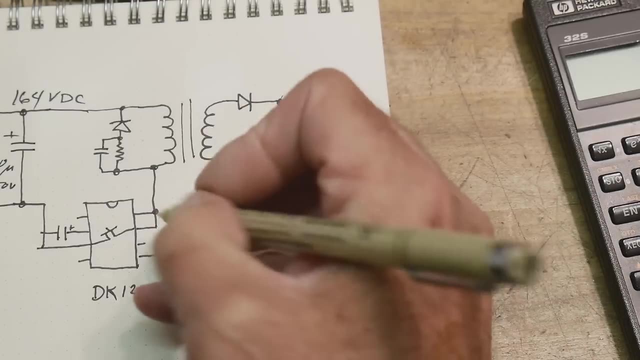 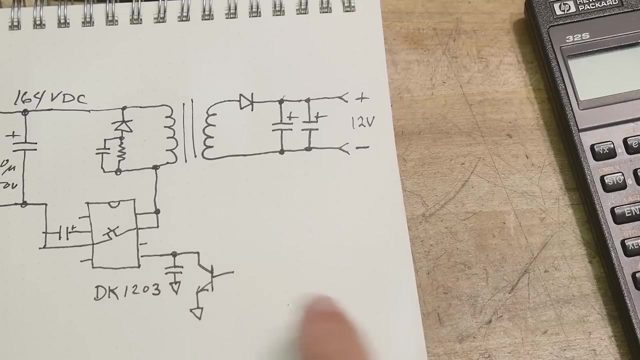 Okay, So this is what the this is what the circuit needs, All right. And then they want to Make that nice, a nice voltage, a nice smooth voltage as well, So they put a capacitor here. Okay, So this is how you regulate this guy with this. 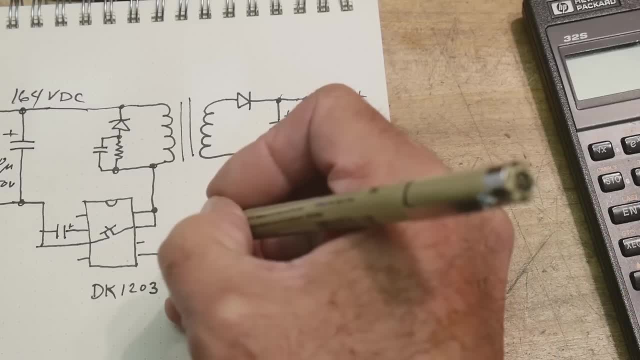 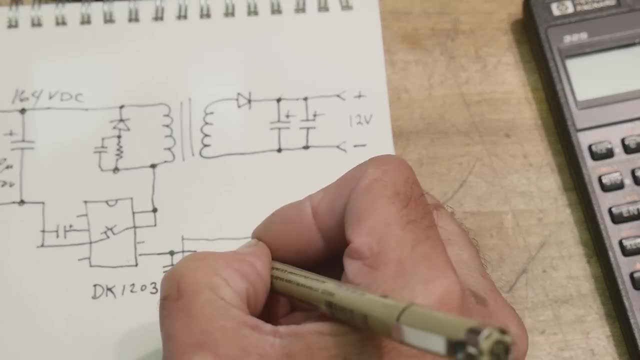 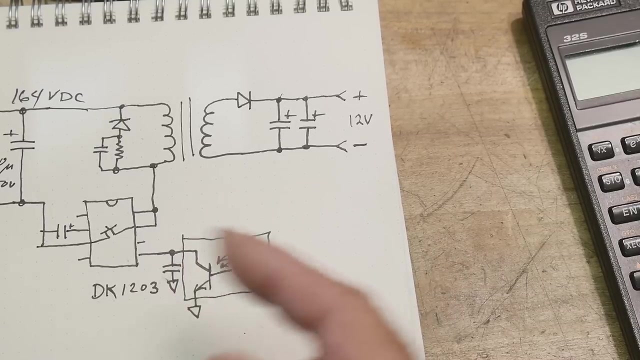 All right, All right, But this we can put in an optocoupler. Okay, This can actually be light, a light photodiode. Okay, An opto, an opto opto transistor, And, And the way that it works is there's a LED over here. 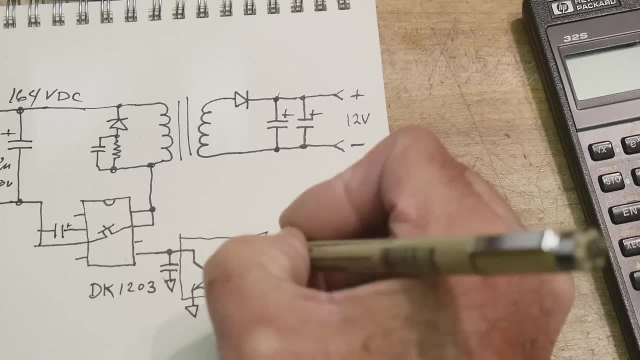 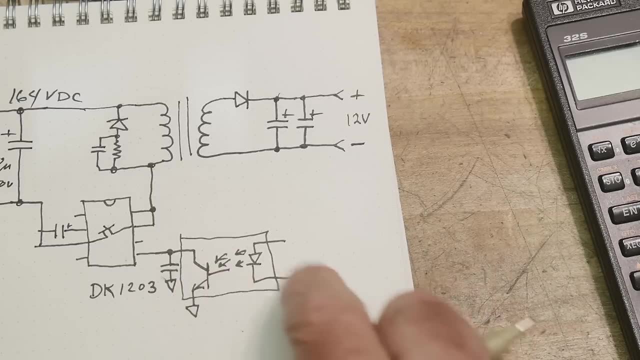 And that LED outputs its light. So when the LED is on, the transistor is on, Okay, And so we can control over here, and it turns it into these optical signals and that'll control over here. So that's how they isolate the two halves. 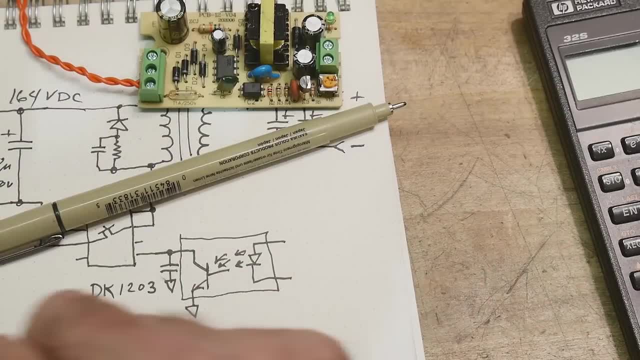 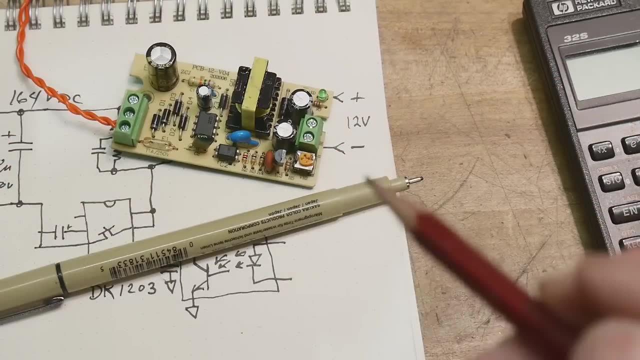 They use an optocoupler. Okay, So the optocoupler. There's my pointer. All right, So the. this is the IC, the, the DK. can I zoom in a little bit? That's all I can do. 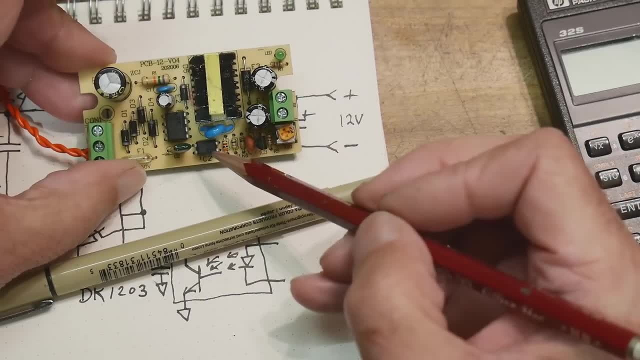 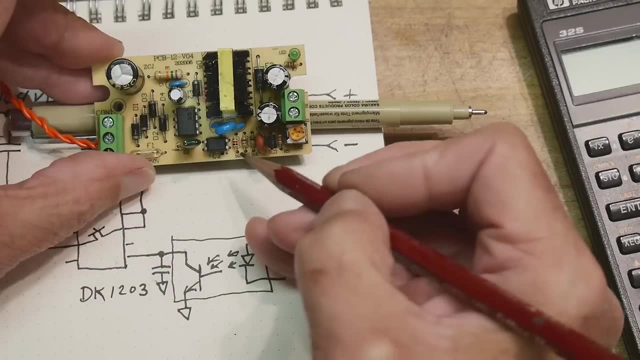 This is the DK1203 and this is the optocoupler right here. This is the optocoupler. It has four pins: Two pins here and two pins here, So the diode's over here and the transistor's over here. 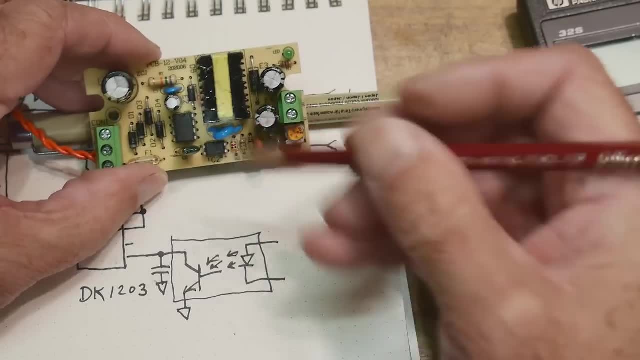 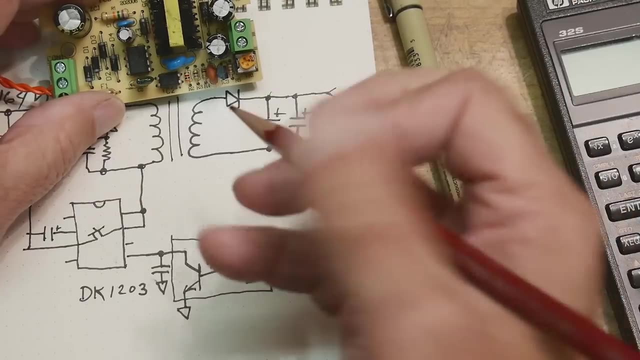 So that is the optocoupler. All right, So now. all we have to do now is figure out how do we get the right signal, How do we tell this guy He's either too too big a voltage or too little of a voltage? 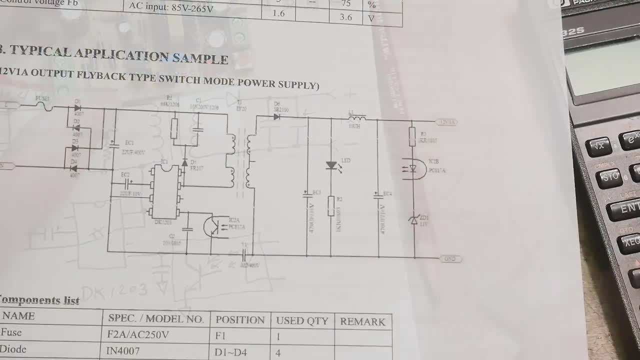 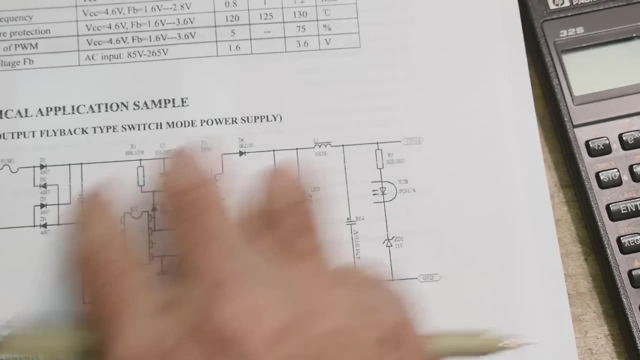 And so let's figure out how to do that, All right, All right. So this is the data sheet for the controller chip, and they give a sample circuit here, And this sample circuit looks almost identical to our circuit. It's pretty much identical on the left-hand side. 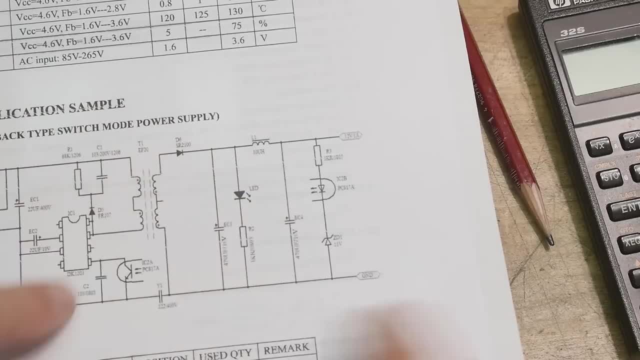 on the high voltage side. It's a little different on the low voltage side. But they tell you how to use this optocoupler. Here's the LED part of the optocoupler and here's the photo transistor part of the optocoupler. 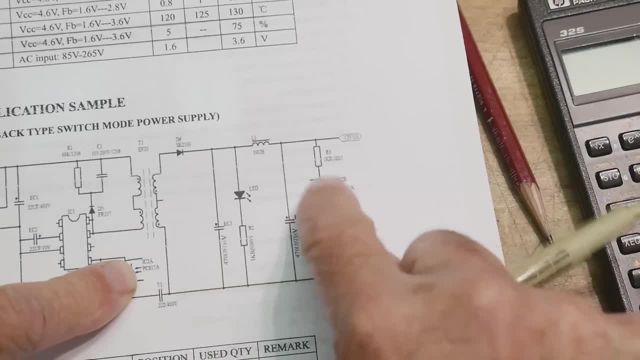 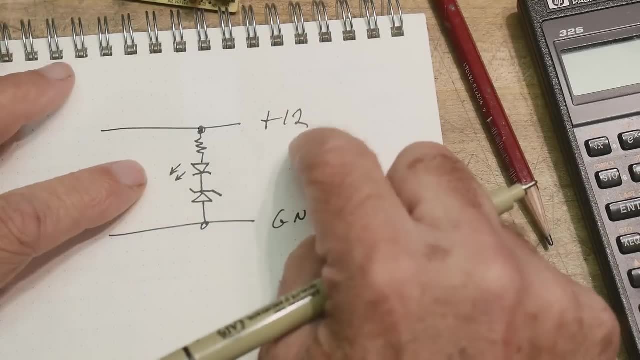 And so we've already drawn this in. But this is how they turned on and off their LED and monitored the voltage, So they wanted to monitor, they wanted to regulate to 12 volts, And so they used an 11-volt Zener. 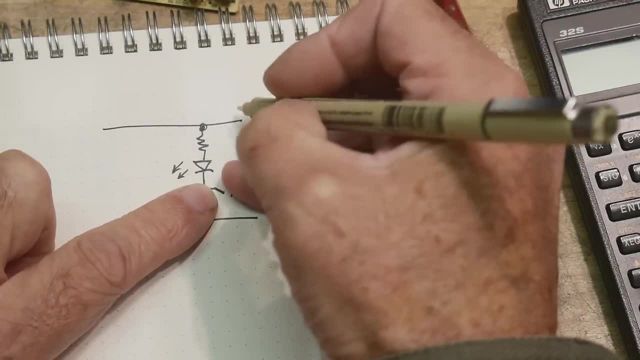 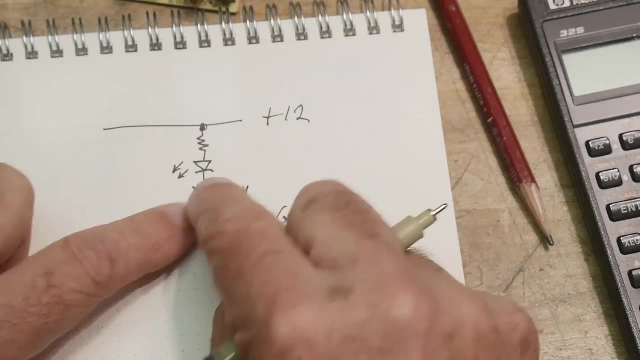 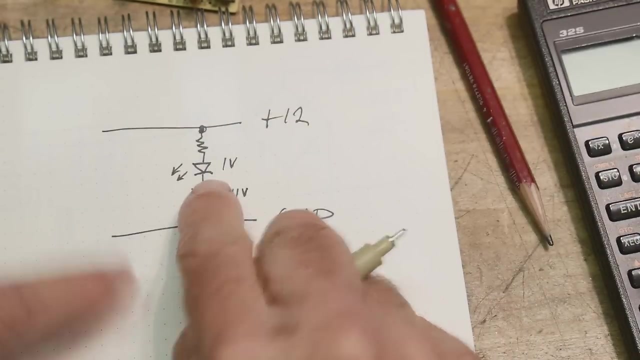 All right. So if this voltage gets high enough, it needs to get above 11 volts and it needs to get above the forward voltage of the LED. So let's say the LED is a 1-volt forward voltage and then you have 12,. 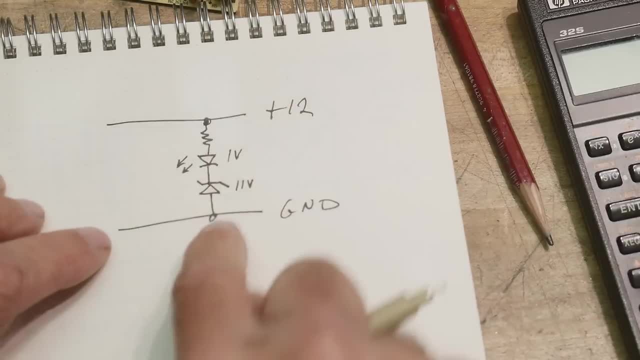 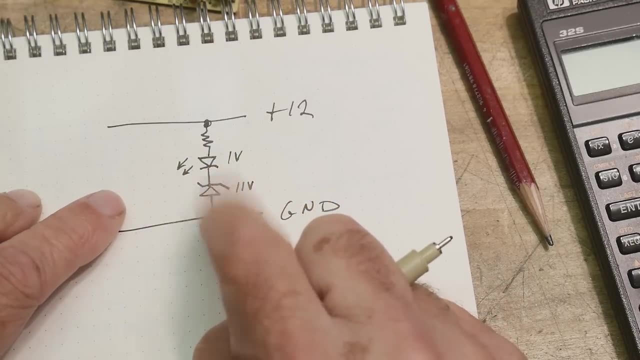 11 plus 1 is 12, you'll get current flow in the system and that LED will turn on. So the higher you go, the brighter that LED will become, And if that LED becomes very, very bright, then it will turn. 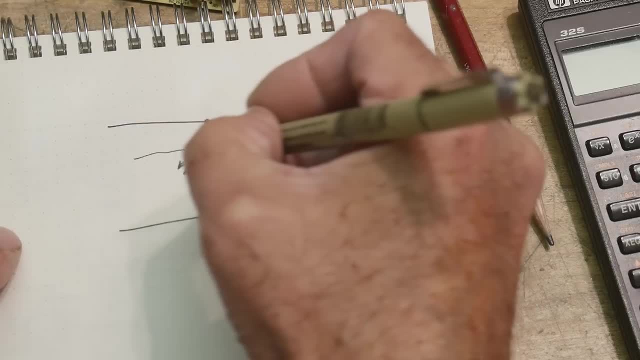 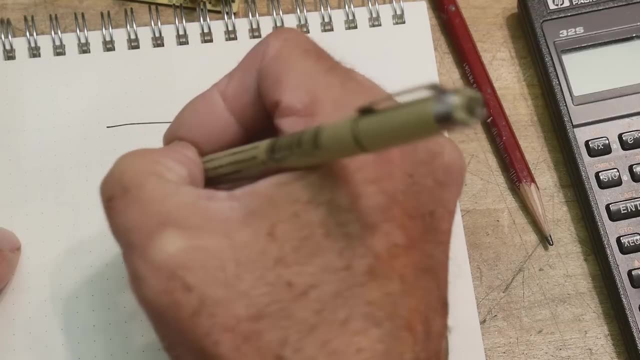 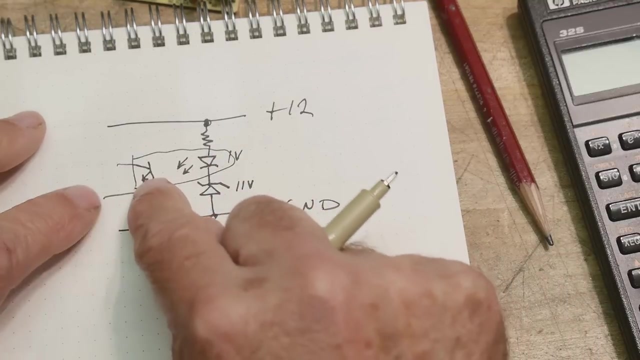 on that transistor in the optocoupler right. This is part of the optocoupler. There's a there's a transistor over here, Remember, And so if it gets too bright, it turns this on harder and harder. 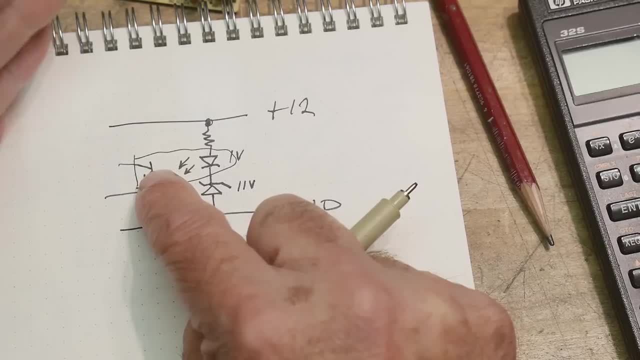 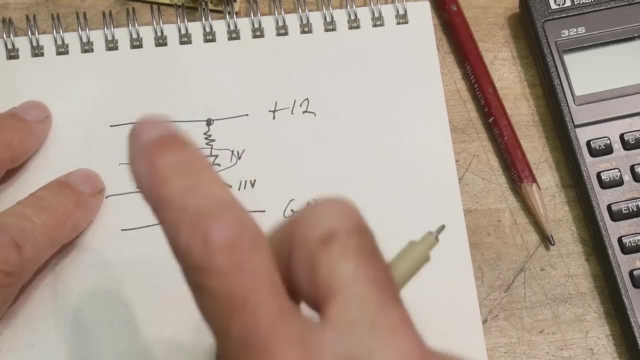 And that will tell the modulator, the, the controller that has the tickle, tickle, tickle thing, to stop right, You're getting too much voltage And that's the way it will modulate. It does a pulse with modulation scheme. 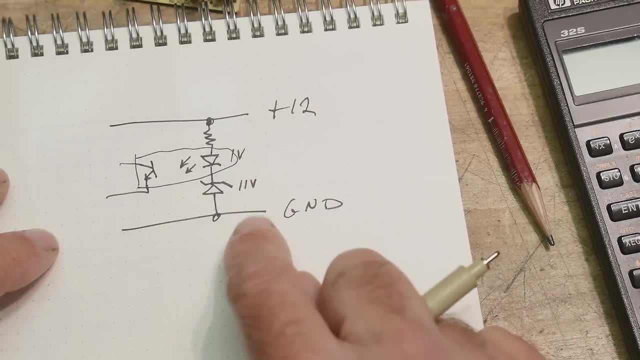 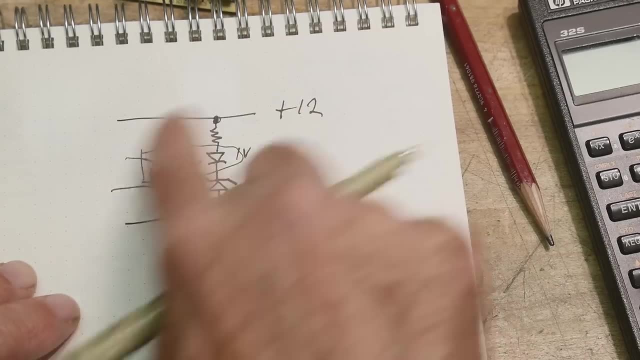 And that's how it will regulate by this method. So this is quite easy to understand, right? 11 volts. if it's bigger than 11 volts and bigger than the forward diode, then it turns on And you can imagine how this, how this works, right? 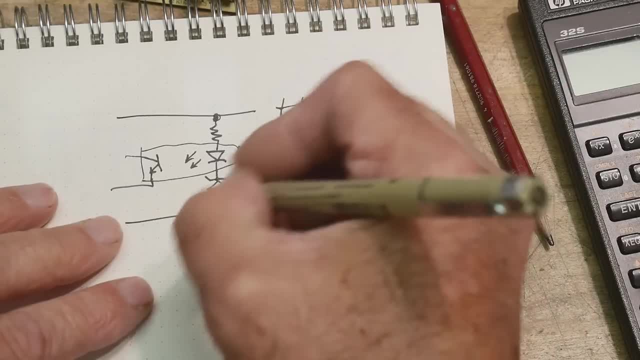 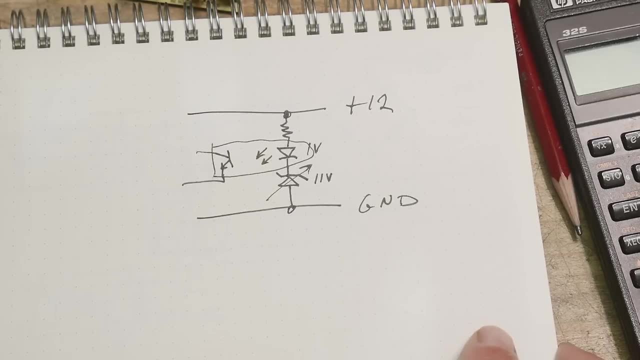 But it's a little hard to adjust right. You kind of would like to have maybe an adjustable zener here or something right, And that's just too hard to do. So they came up with a clever circuit, And the circuit's a little bit complicated. 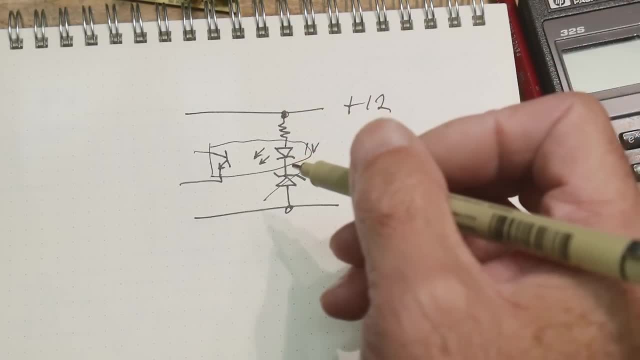 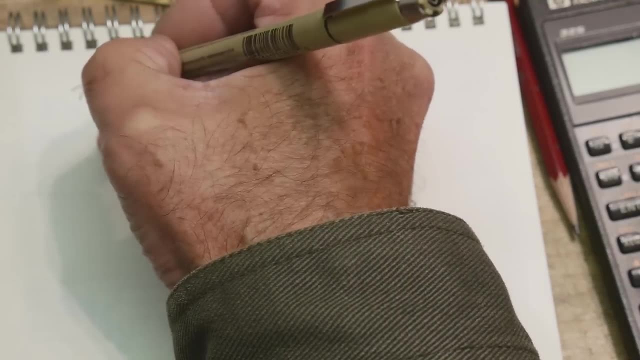 But if you remember in- I don't remember which video it was in- I talked about a TL4.. I don't remember which video it was in. I talked about a TL4.. 431.. And it was a funny part. It looked like a zener diode. 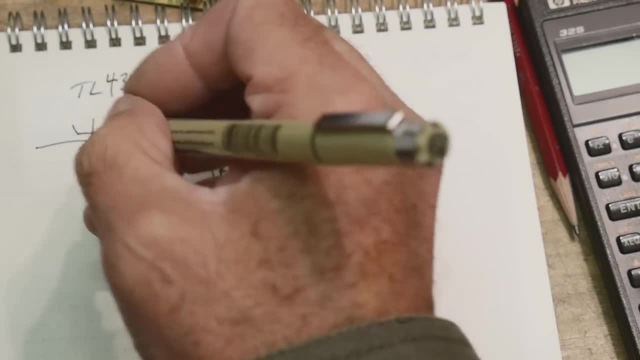 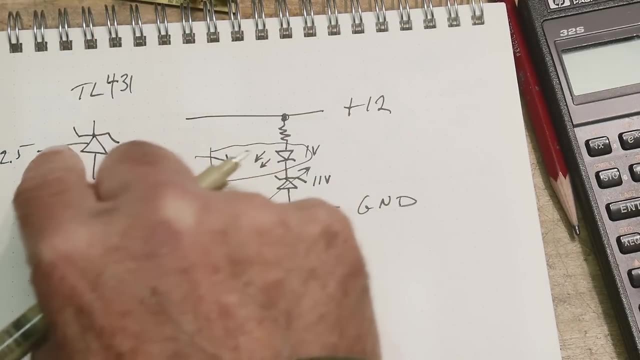 But it had a control pin on it, okay, And it was like 2 1⁄2 volt device. It wanted it wanted this control voltage to be 2 1⁄2 volts If this was ground and this was 2 1⁄2 volts. 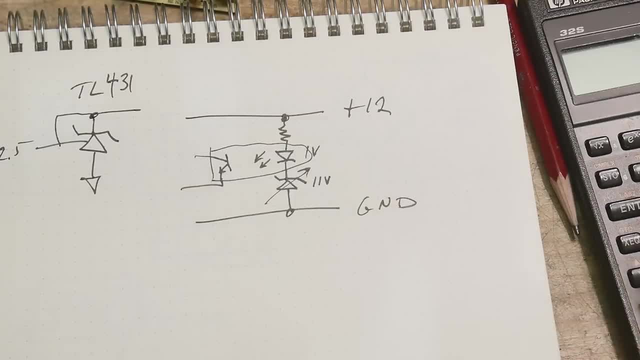 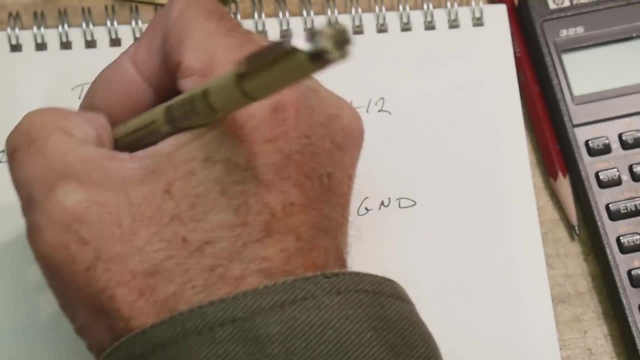 if you tied these together, the output would be 2 1⁄2, okay. But if you put a divider here, if you put a resistor here and a resistor here, and these were both the same resistor, then you'd get 5 volts out here. 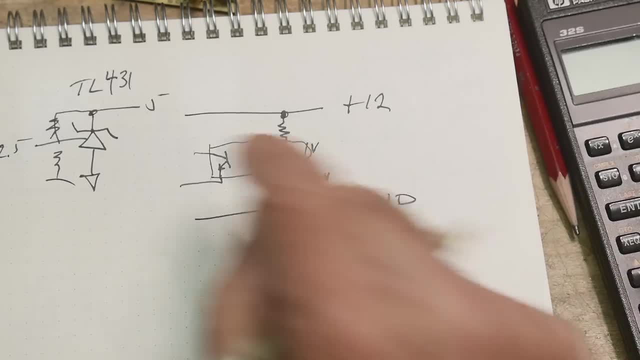 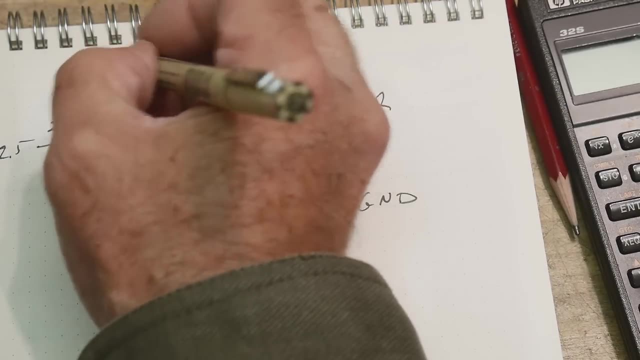 It did whatever it needed to do in order to get this 2 1⁄2 volts, And so this particular circuit uses a TL431.. Now, that's a very, very stable part, And so you have a good voltage reference in order. 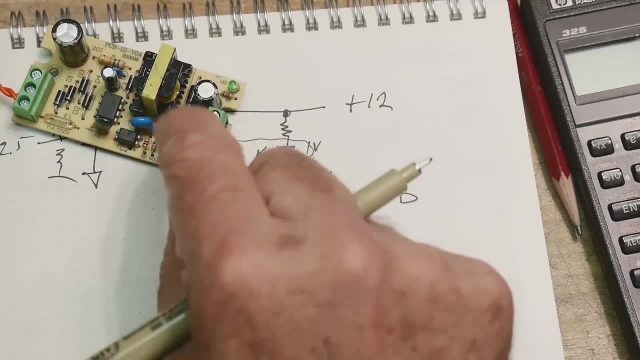 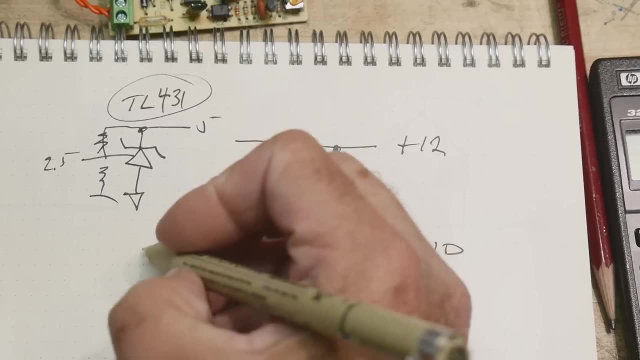 to control this. So this will be able to be tuned in very, very accurately And we'll draw this circuit and I'll show you how that works. Okay, So we're going to use this part in a little bit of a strange way. 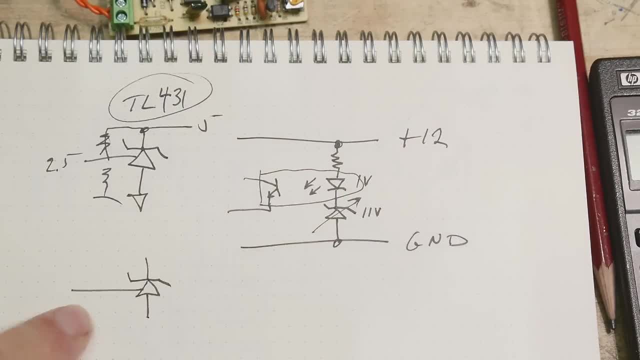 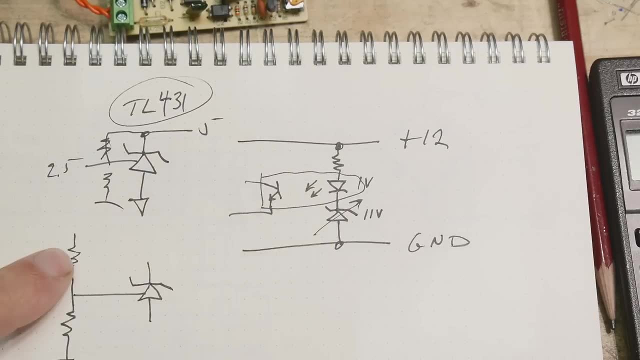 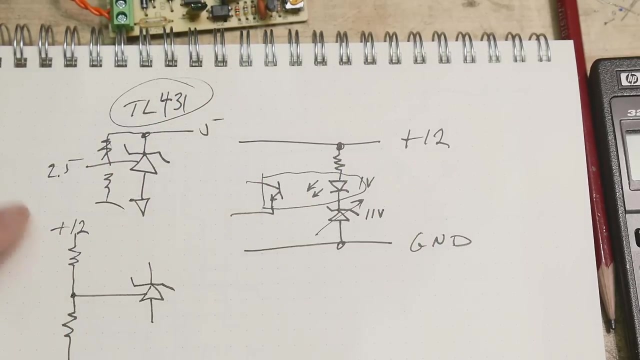 We are going to use that control pin and we need to put 2 1⁄2 volts on that control pin, okay, And we're going to be monitoring our 12 volts, okay. So we need a resistive divider that gives us 2 1⁄2 volts. 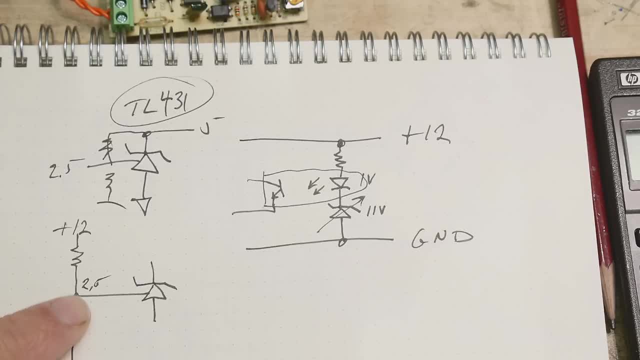 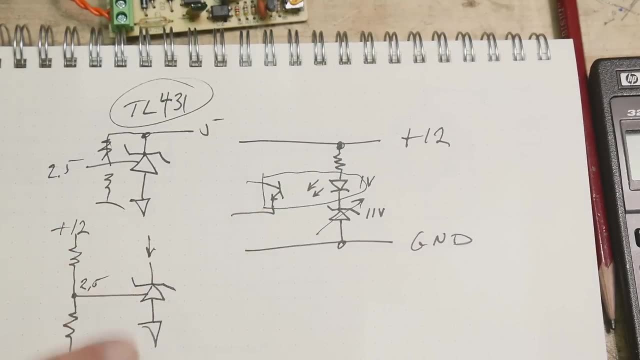 Now, if this 2 1⁄2 volts gets a little too high, it will start drawing current through this device, And if it glows below 2 1⁄2 volts, then it will stop current in this device. 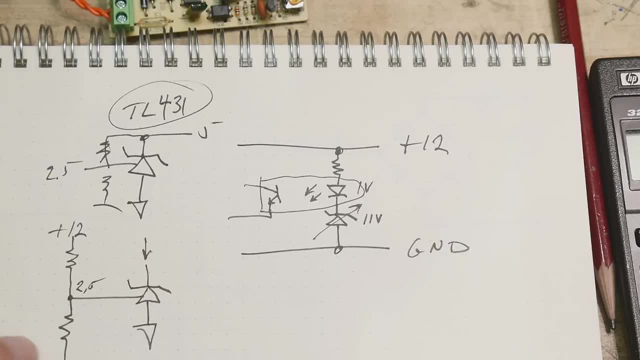 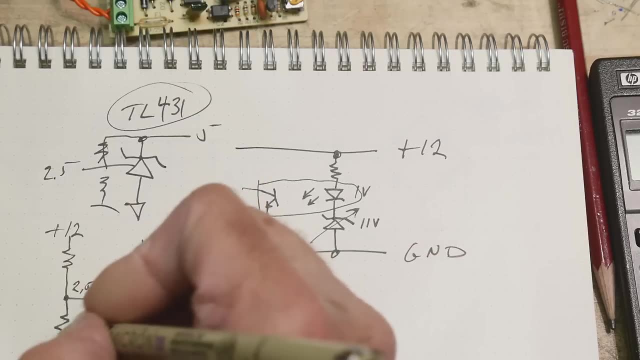 So that's the way this is going to operate. So you can see that we're going to have this divider on our 12 volts and we're going to be able to set this 2 1⁄2 volts. In fact, one of these is going. 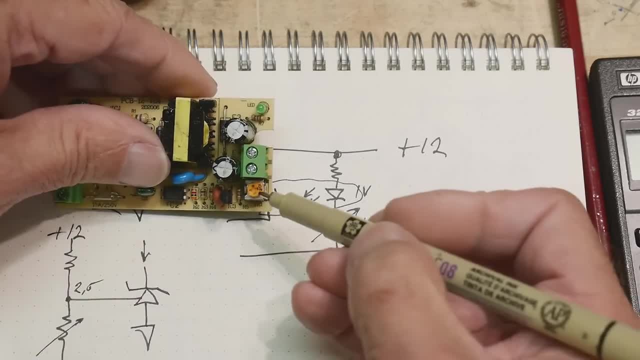 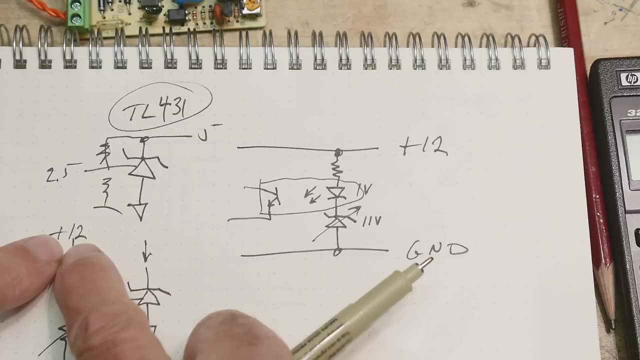 to be a potential And that's right down here. That sets our voltage, We can adjust it and that will be here. So this resistive chain, all its function, is to take our 12 volts and regulate it to 2 1⁄2 and do. 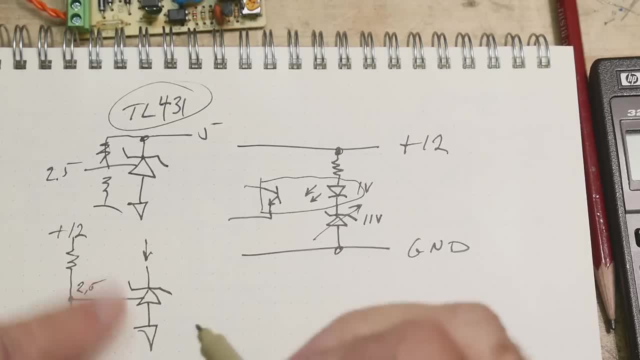 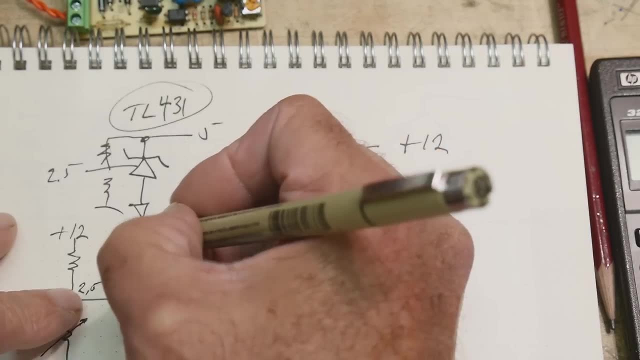 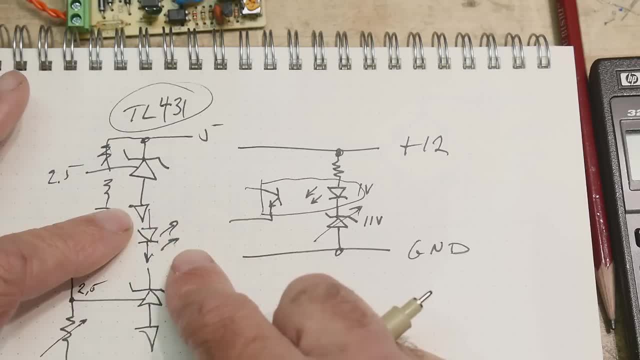 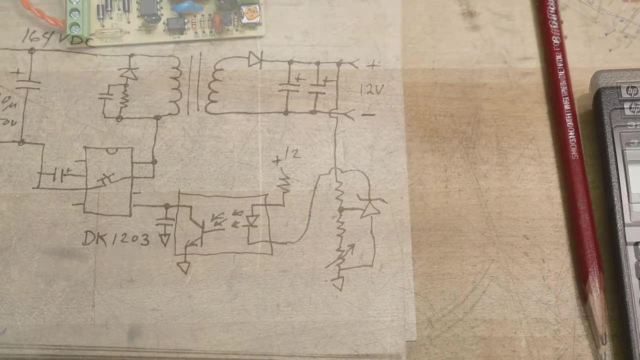 So if this thing starts to conduct current, our LED will turn on. Okay, And so that's what the circuit looks like. So let me see if I can draw in the circuit. Okay, I didn't draw it the best way I could. 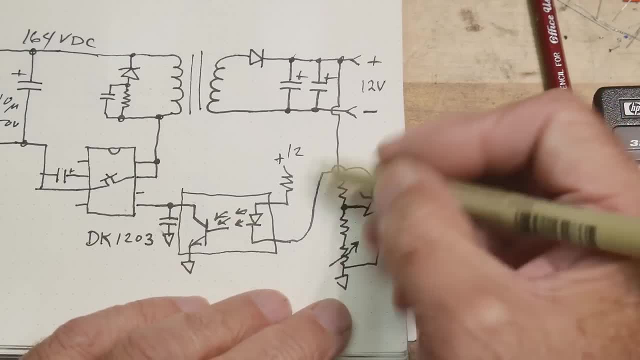 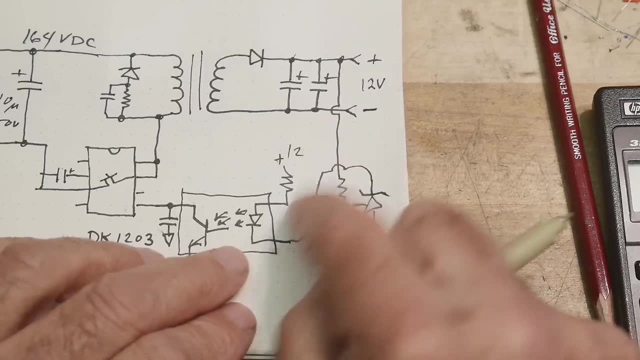 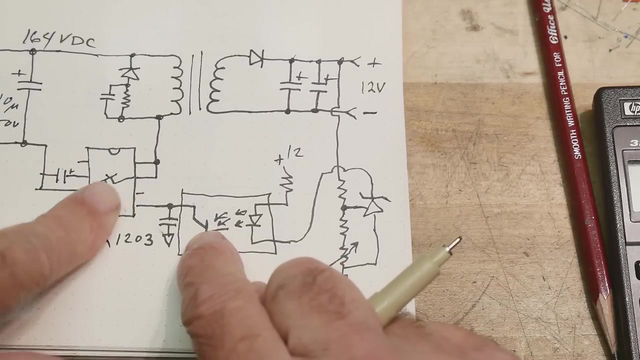 but I did fit it on the page And it's not too important to understand exactly how this thing works. It's. what's really important to understand is that this is how the regulation happens: That somehow you turn this LED on, It turns this transistor on and this thing stops pulsing, right. 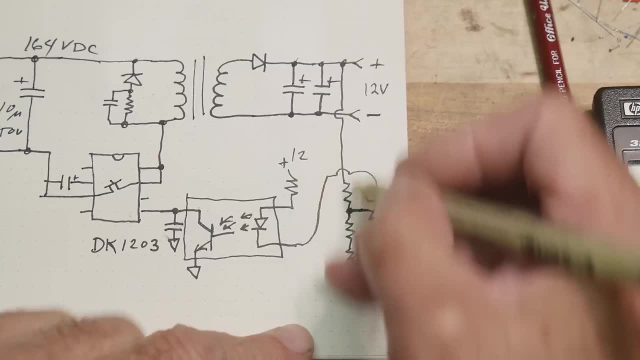 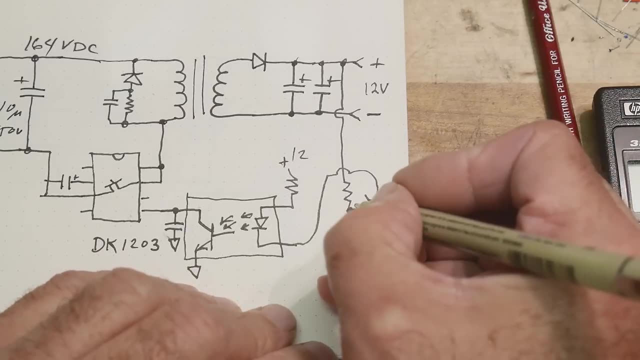 And so the way that we're going to do that, we're going to set up this voltage chain here. This goes up to the 12 volts. So we have these two resistors and then a potentiometer, and that allows us to fine tune this 2 1⁄2 volts. 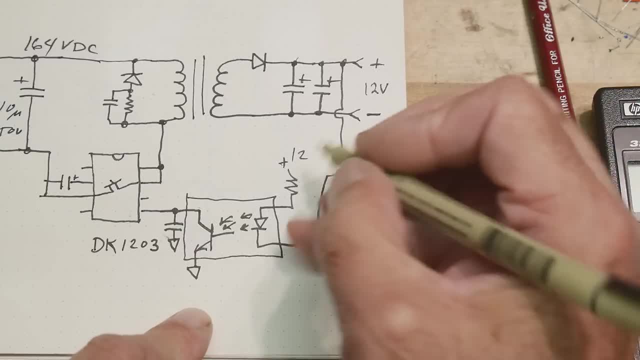 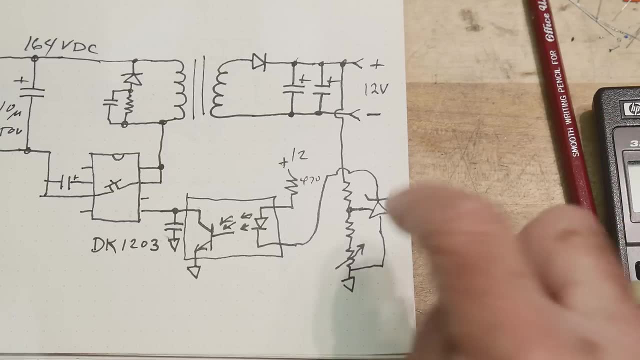 And then the LED has a little resistor in it- I think it's a 470 ohm or something like that- And then it goes through the LED and then through this TL431 and then to ground. So that's how the LED gets turned on. 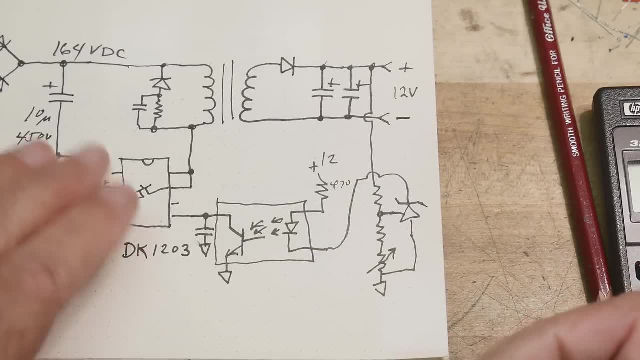 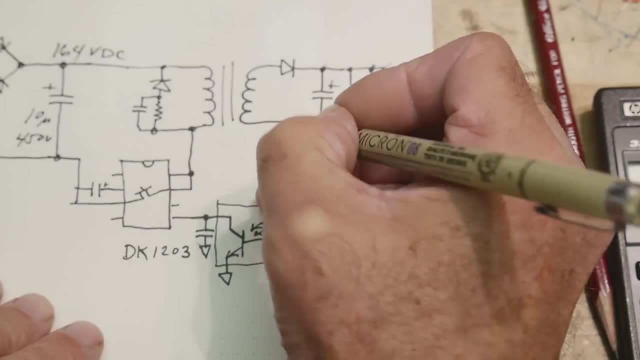 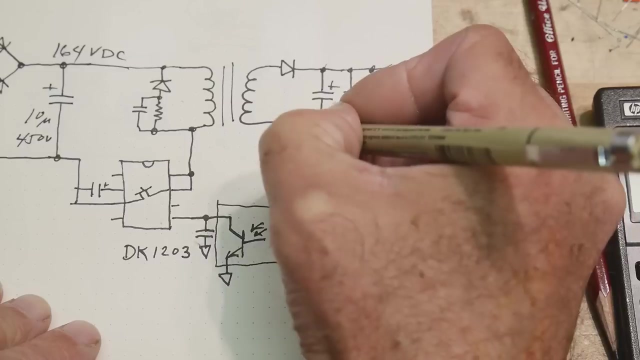 It's turned down. So that's it. There's only one other thing in the circuit, and that is that there is an on LED and there is a LED in there. Oops plus 12. The LED goes in this way and goes to ground. OK. 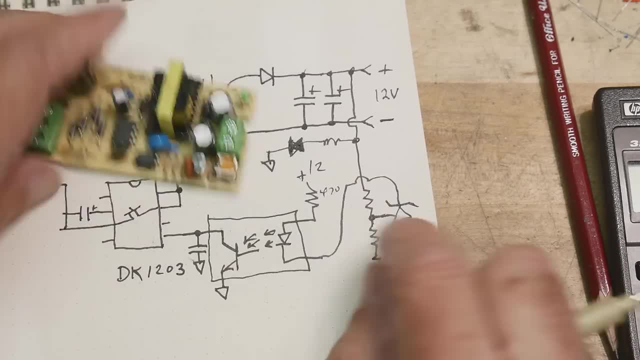 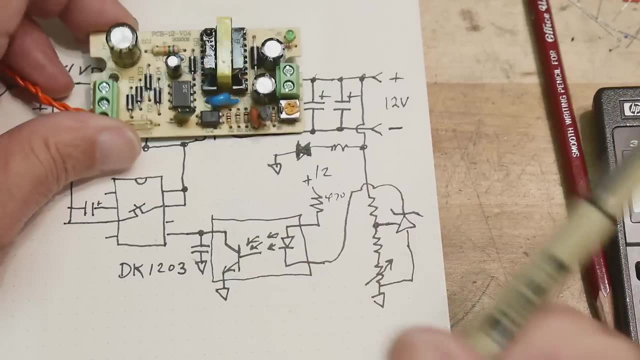 So there's an LED and that is all that is on this board. OK, Well, there's one part left. One part left, OK, OK, But everything else Actually covered everything on the board now, except for this one blue capacitor, and we'll talk about it later. 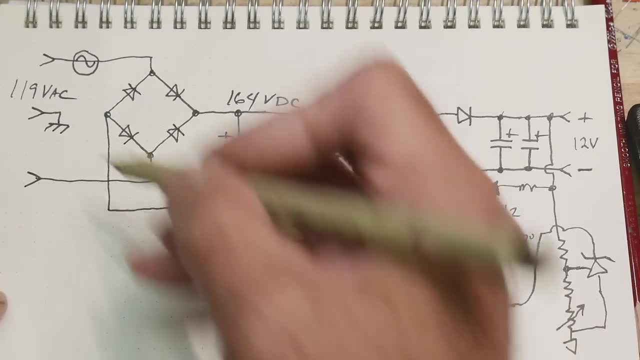 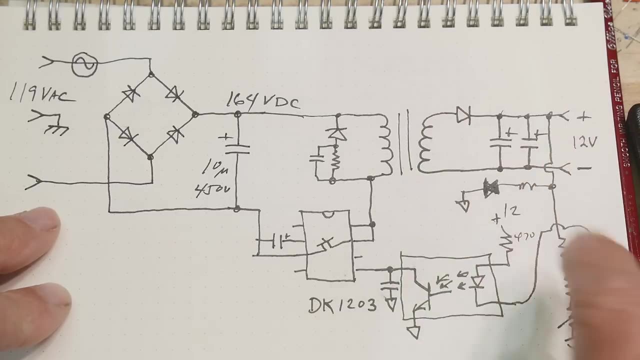 So I hope you understand everything. now AC comes in, It gets into a high AC and then we're going to turn it into 12 volts over here. OK, So we're going to need, you know, somewhere around 12 volts here. 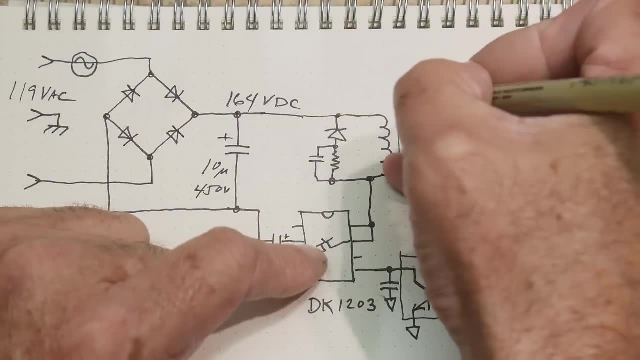 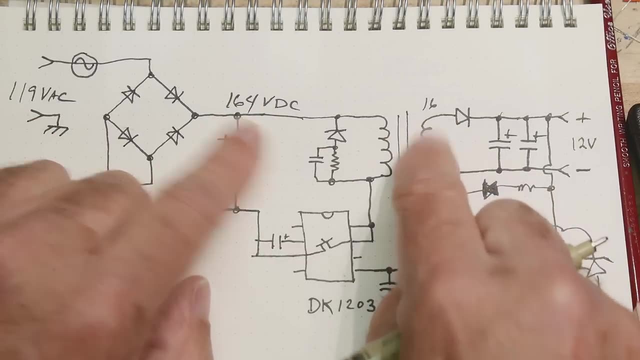 And so you can see that if we need, let's say this is 16 volts AC here, and then we rectify it down to 12 or something. We have 160 volts here, We have 16 volts on this side. So this transformer has to have about a 10 to 1 wind ratio. OK, 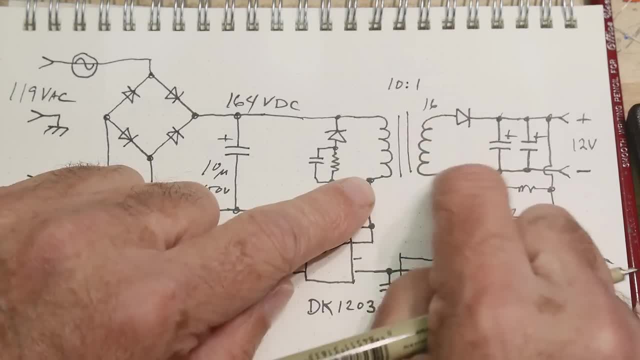 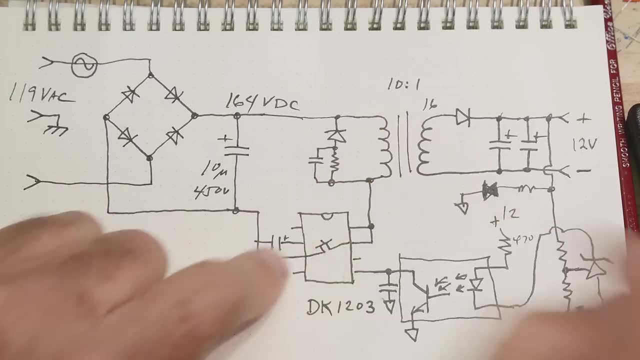 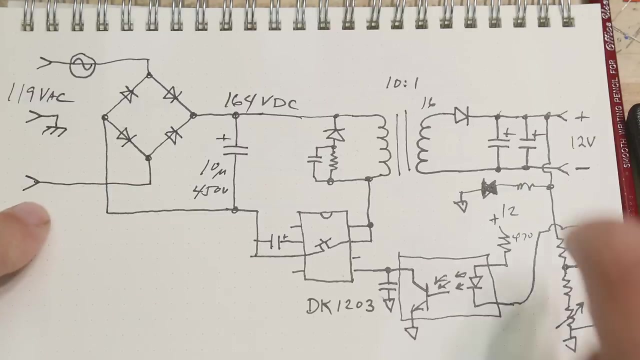 There's going to be 10 times more windings on this side than this side, And this 10 to 1 transformer takes us from this high voltage to this low voltage, And so AC, DC, AC, AC, DC, and then the DC is monitored. 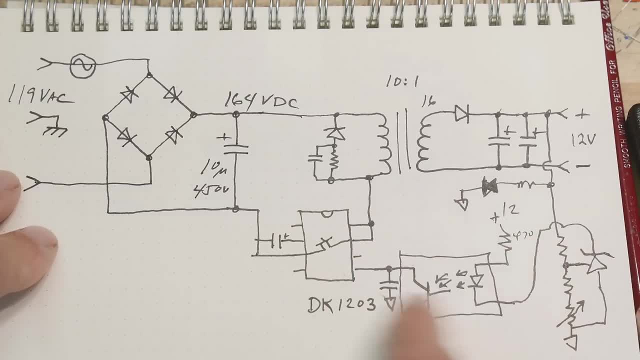 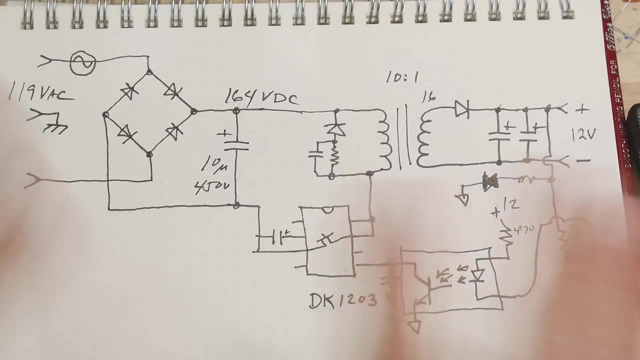 and then it's communicated to this chip with this optocoupler. hey, you're either too high or hey, you're either too low. You know, pulse some more because you're too low, or don't pulse as much because you're getting too high. 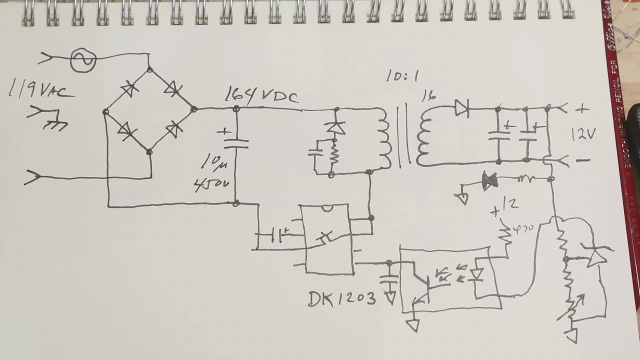 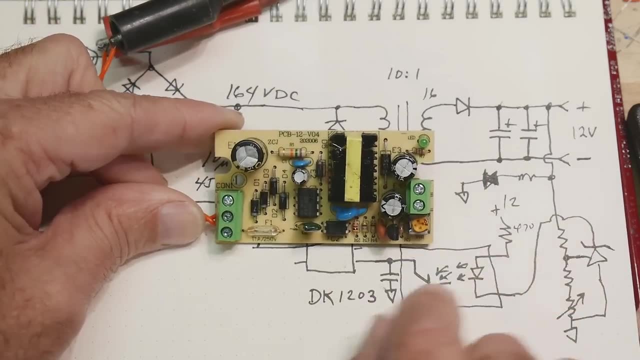 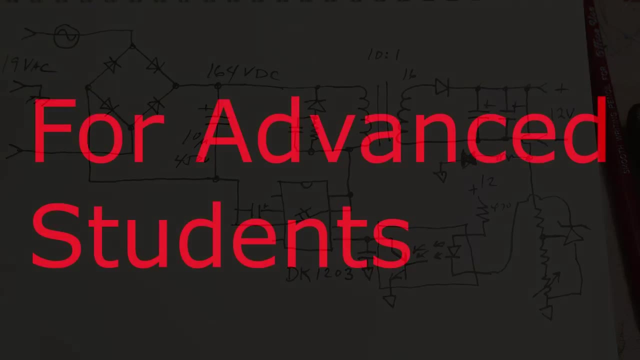 And that's it. That's all there is in this thing. So it's a nice little first circuit to look at for switching power supplies and get to the idea of what's going on. So I hope that helps. So we have one component left to go. 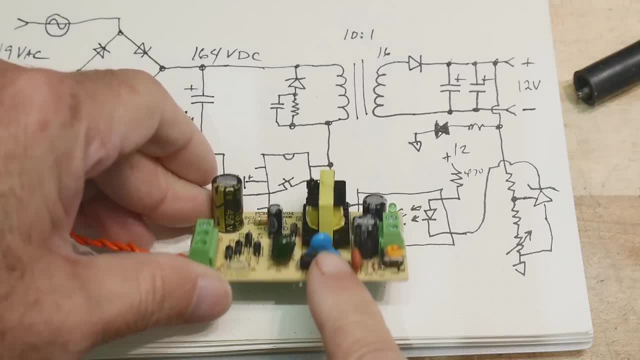 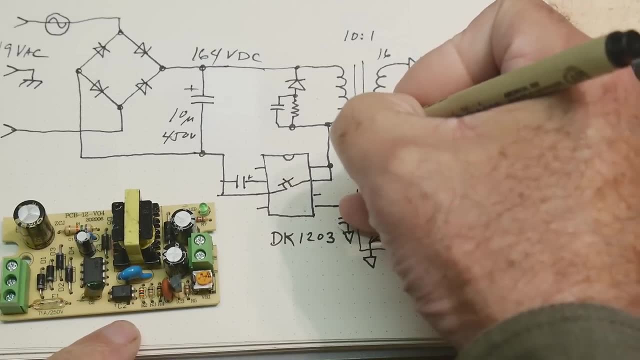 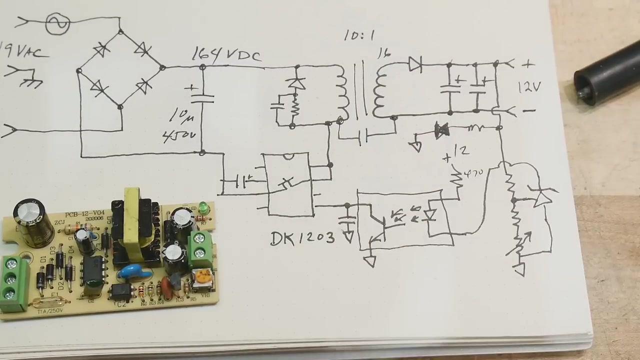 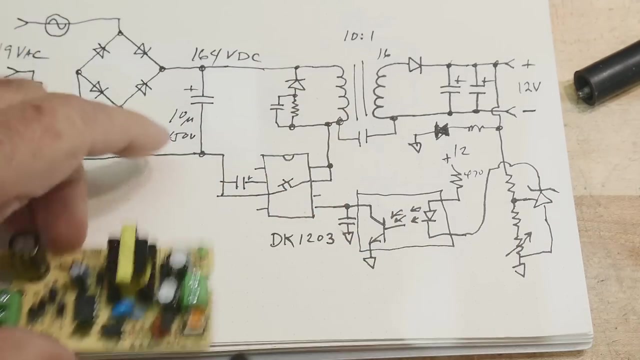 and that is this strange blue capacitor. What is that blue capacitor doing in there? Well, that blue capacitor goes right here. It goes across the transformer. So you can imagine the transformer windings are kind of being in proximity to one another, right? 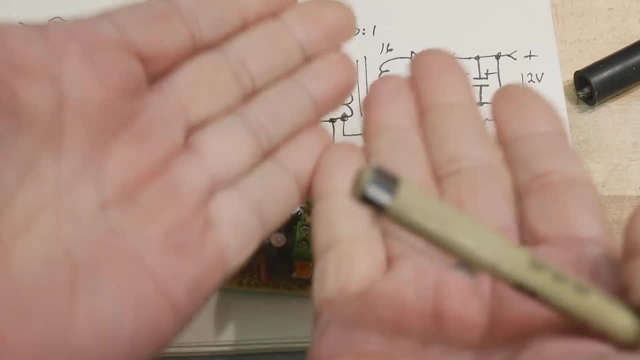 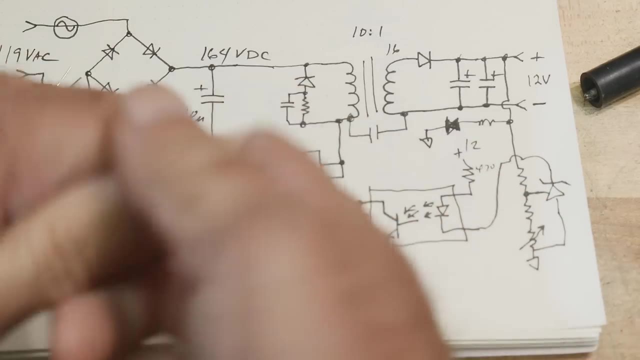 They're all wound around the same core, So there is some. when you put two wires together- I showed this in one of my videos, I called it a mimic- You take two wires and you spin them together, You get like a five picofarad capacitor. 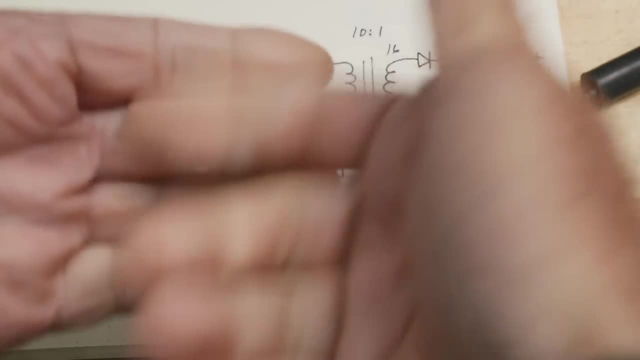 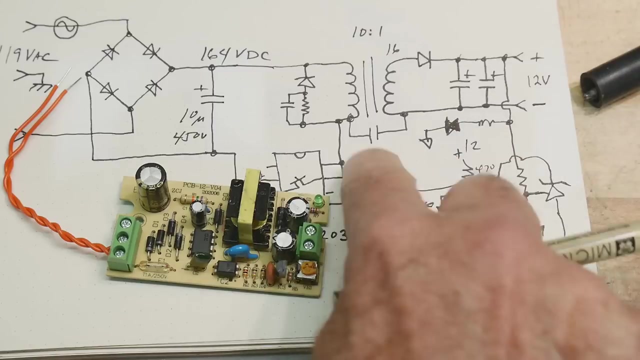 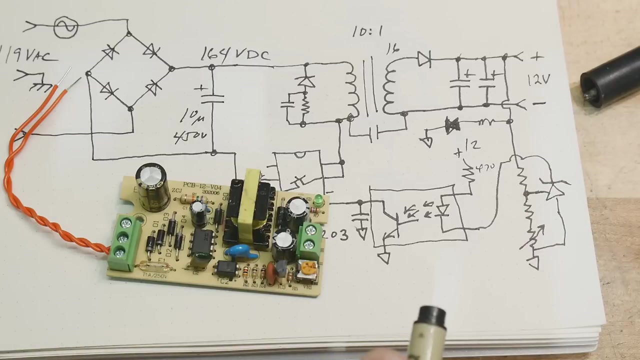 And if you look at wires close together, they're going to have some capacitance across each other. And what does that capacitance do? Well, it lets signals pass. It lets high frequency signals pass And it also stops any signals that you want to have grounded. 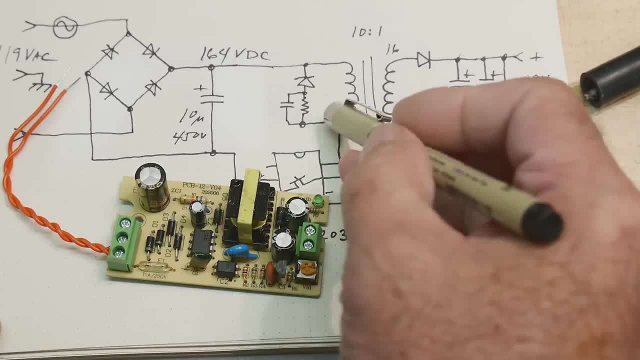 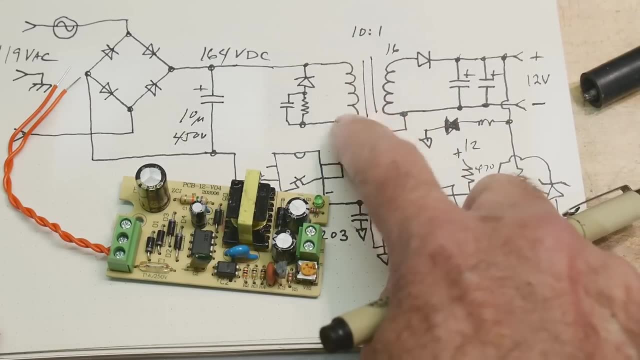 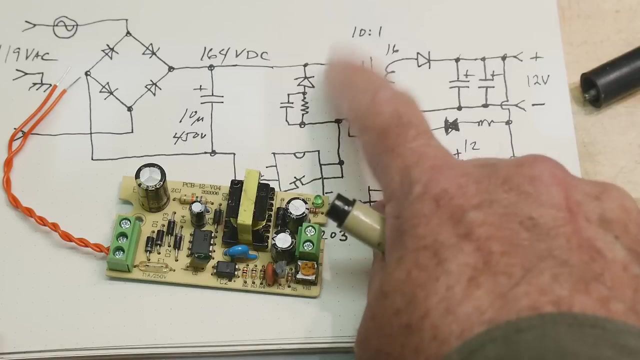 So if you have ground on one side and you need a high frequency path to ground on the other side, it'll short those out. That's what this does. This is a high frequency capacitor that allows these high frequency spikes to be snubbed. 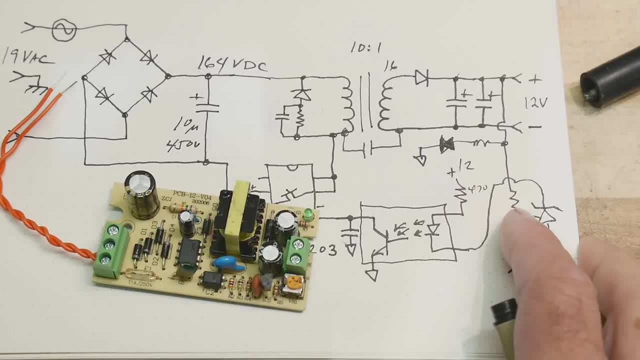 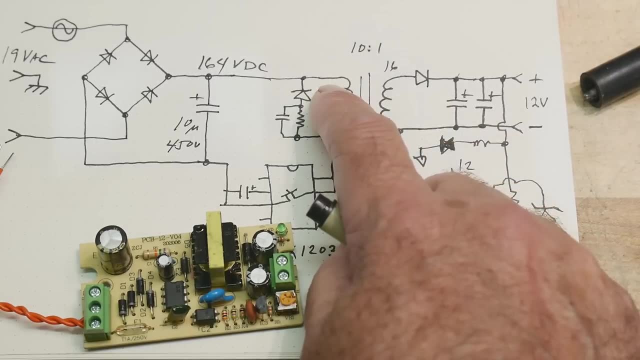 Well, you can kind of think of this as a snubber too, but for a different reason. This side is going to create a whole bunch of high frequency noise, And that high frequency noise is going to go every which way, And so it's found that 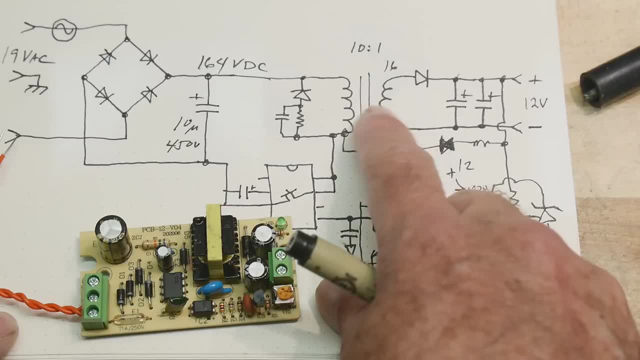 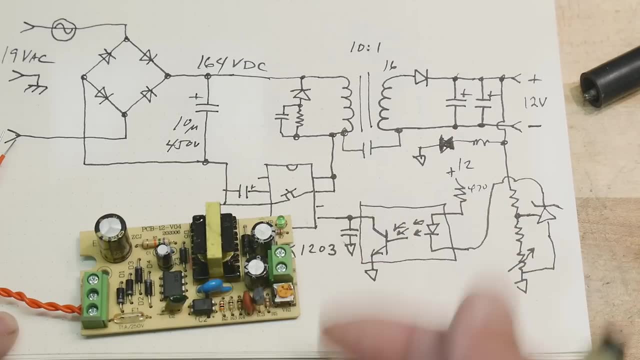 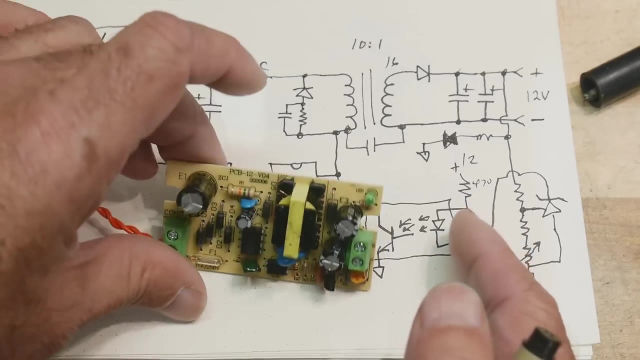 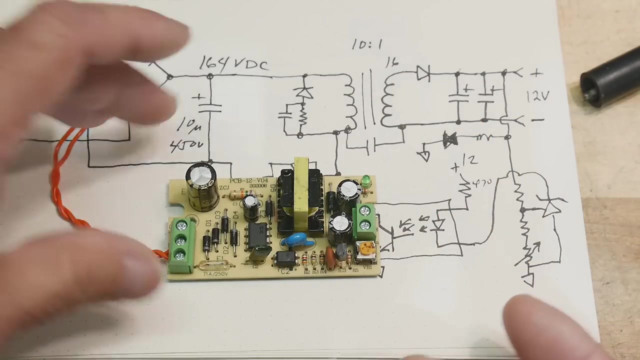 by putting this capacitor in here and shorting out any high frequencies between these two coils, you can lower the EMI, which is the radiation of this RFI radiation of this device. So without that it would be noisier, It would output more radio interference waves. 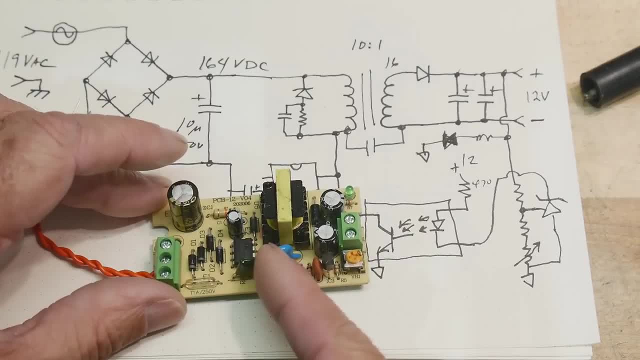 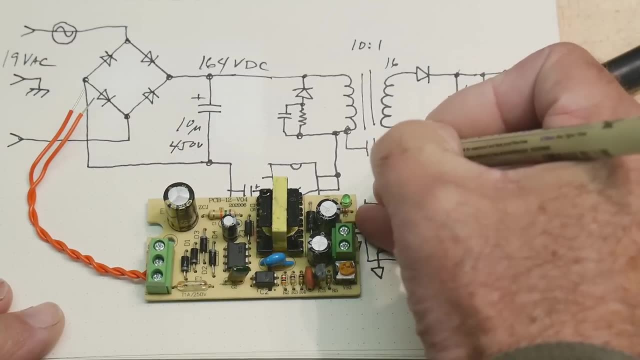 than having that in there. So that's why it's in there, And it has to be a high voltage capacitor and it has to be AC rated, And so they use a Y capacitor. I don't know why they don't use an X capacitor. 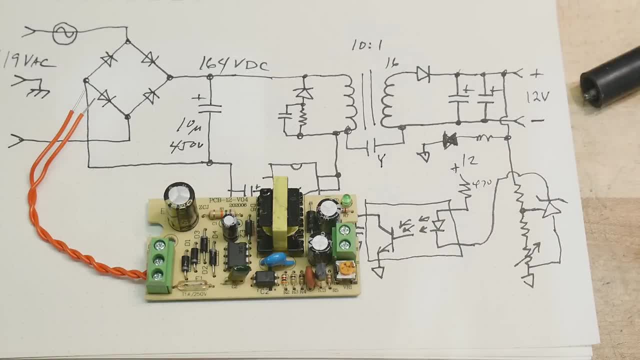 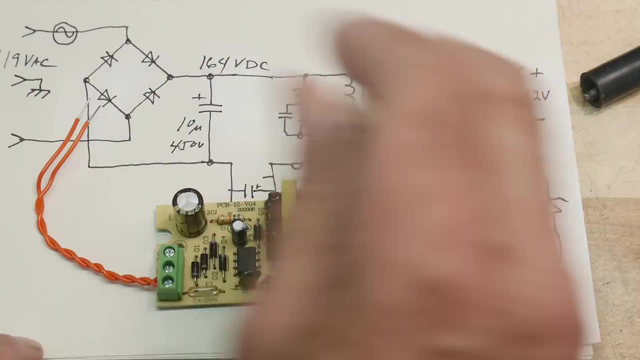 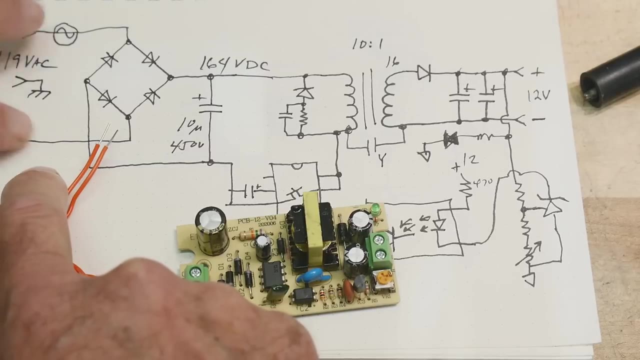 but they use a Y capacitor. So Y capacitors are used to to filter the input from RFI situations. also, They're generally put on the AC lines to ground, So there'd be a capacitor here to ground and a capacitor here to ground. 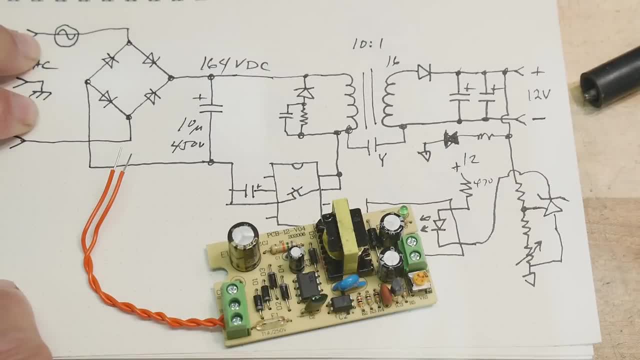 You'd have these two ACs, That would be a Y capacitor, And then you could also put one across the two ACs directly, and that would be an X capacitor. So yeah, I don't know. Anyway, that's what that one does. 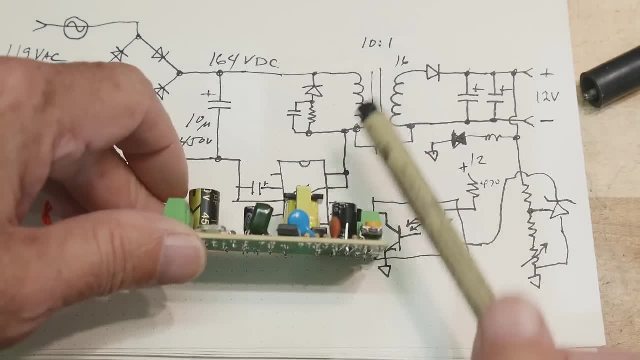 Um, I don't, I don't really have a good gut feel why it works, Uh, but uh, that's why it's in there.